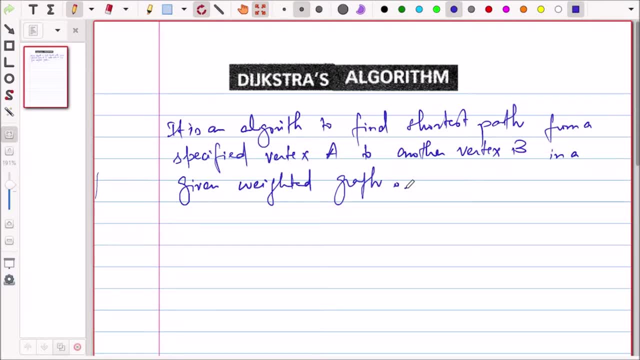 So we can give any value to each of the edge. So what is the simplest value to give? To give one. So by giving one to everyone, we can apply this algorithm there as well. Extra algorithm: Okay, So it is an algorithm to find shortest path from a specified vertex A to another specified vertex B in a given weighted graph. 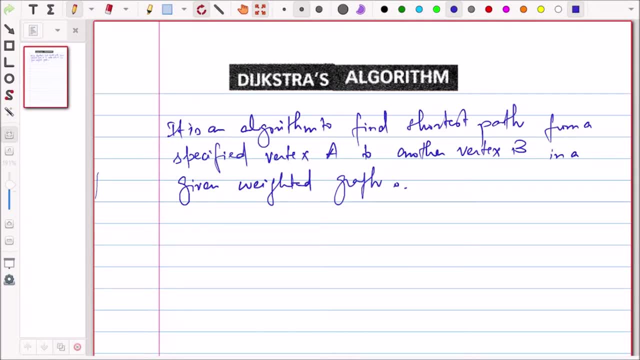 Okay. So what we do is, if in this it proceeds, It proceeds Okay, By progressively assigning. By progressively assigning, Progressively assigning means we are assigning one in one step, So as the steps are progressing, we will assign each vertex. 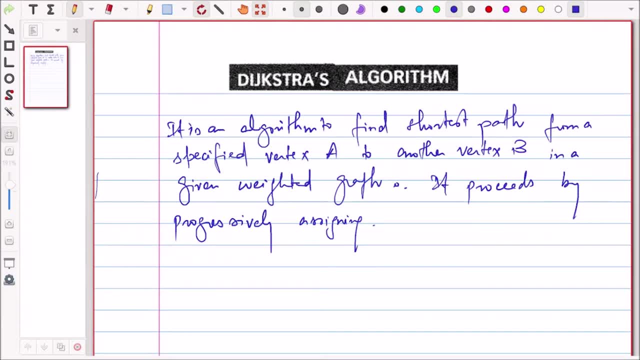 Progressively assigning to each vertex B in the graph, To each Don't Kansas Vertex, The second vertex, Vertex v In the graph. In the graph, An ordered pair. An ordered pair. Next D: okay, an ordered pair. 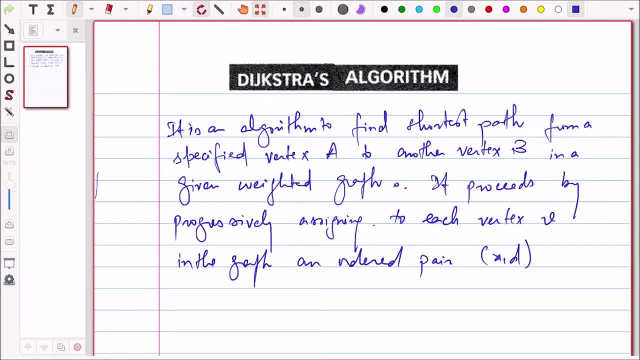 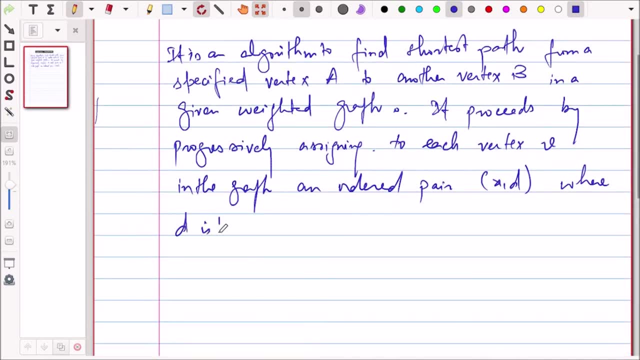 X, where Before D is the Shortest Distance From A to V. OK, D is the shortest distance from A to D And XV is the last edge on the shortest path. And XV is the Last. 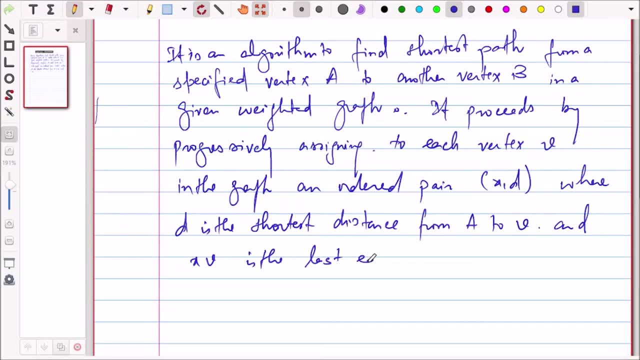 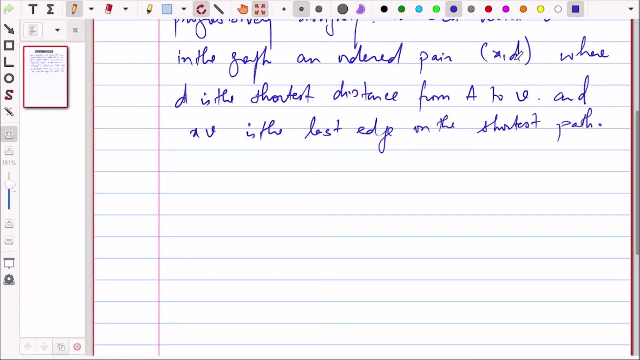 Last Edge on the Shortest path. Basically, X denotes the previous vertex, The previous vertex on this path, And D denotes the distance. OK, Are you getting my point? XT is like a graph. OK, Suppose this is one graph. 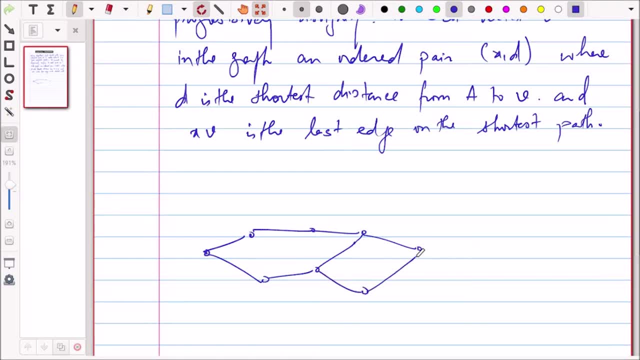 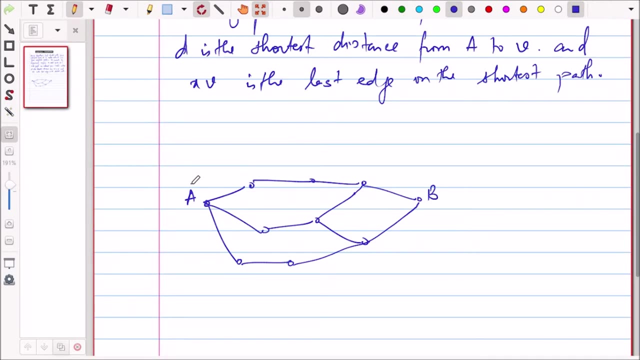 OK, And OK, Let me. So this is our A, This is our B, And let us call gives. So what we do is Now, because this is initial, So there is no one before this, So we will keep it empty. 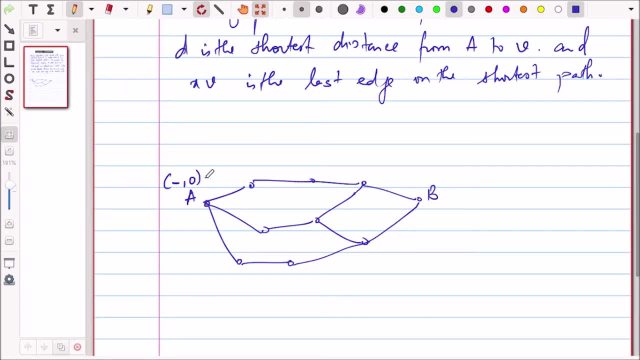 And its distance is also A to A is 0.. This is the distance Right. This is 2.. This is 3.. This is 1.. This is 5.. This is 6. 2. 1.. 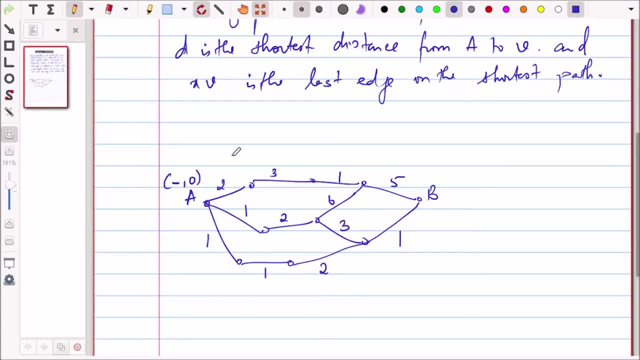 1., 1., 2., 1. 3.. So these are all weights. OK, Now, If we come to this vertex from A, What is So what? its distance? Yeah, Distance A to this Its. 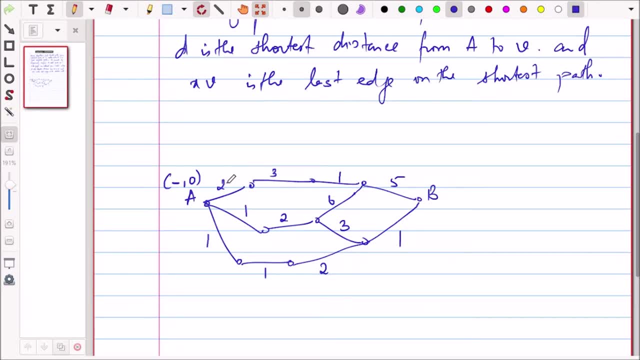 Yes, Yes, The vertex is: It is 2. Right, And the previous vertex from it: Yeah. So we'll label this as a 2.. Similarly, we will label it as a 1.. We will label this as a 1.. 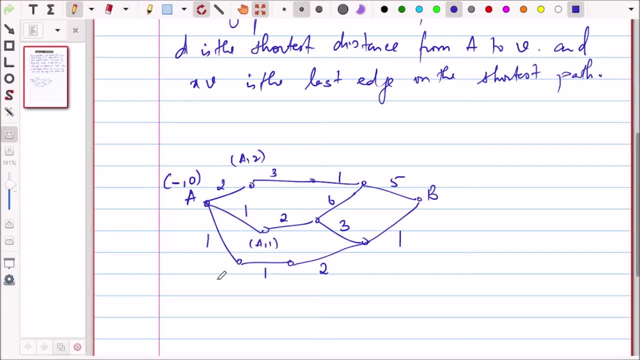 OK, Now we will come to the next step. Now, this is the way to come to this, So we will label this as 2 plus 3. 5. So distance from A is 5. And the previous vertex is this vertex: 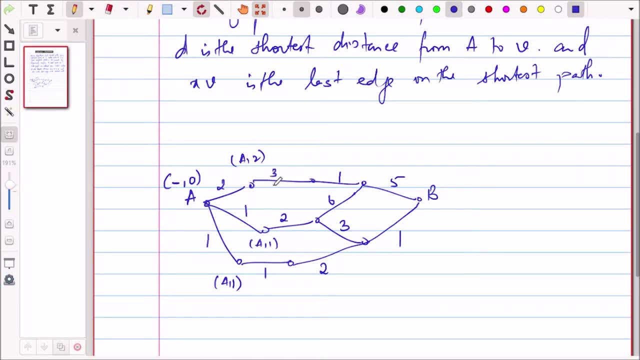 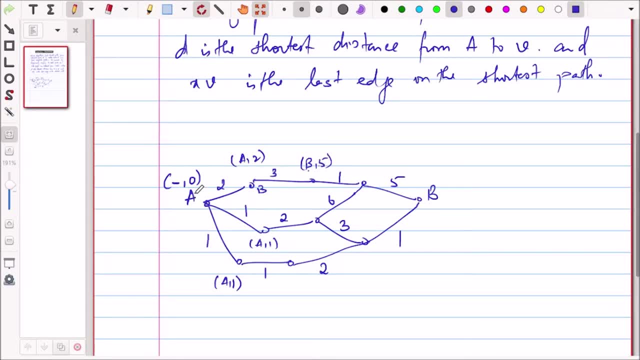 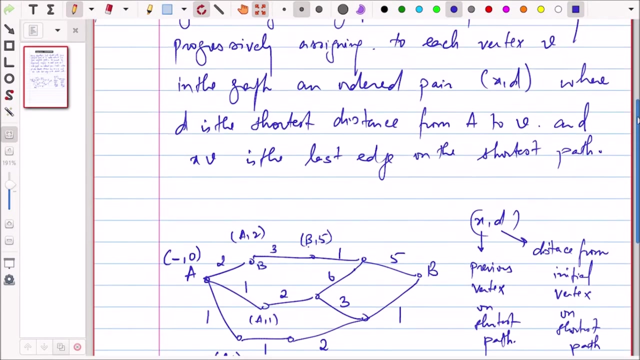 the previous vertex, and five denotes the distance from the initial vertex. okay, so extreme a distance from initial vertex. initial vertex on shortest path. and x denotes previous vertex on shortest path. okay, is it fine? okay, so now, let us, uh, give you the. let me just give you the. 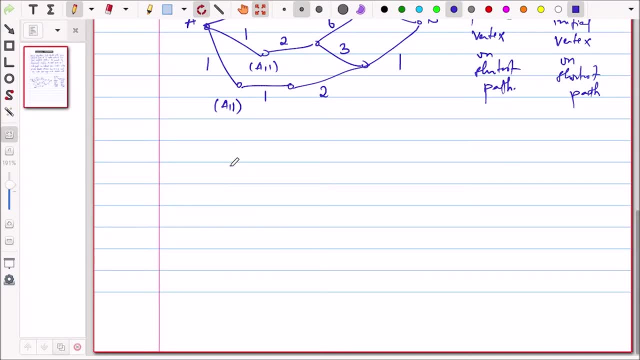 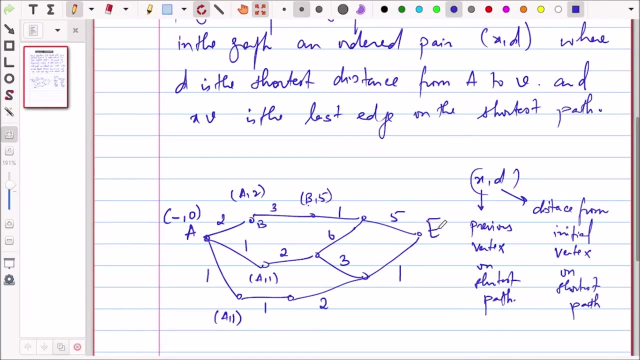 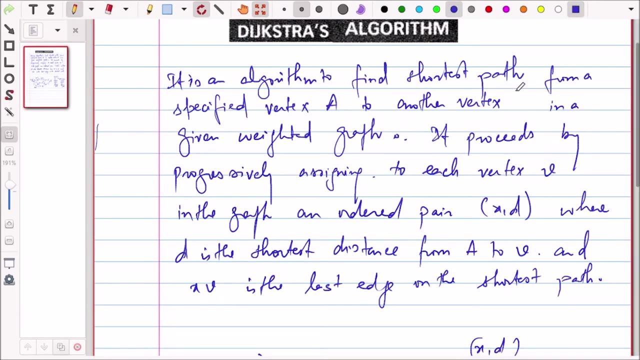 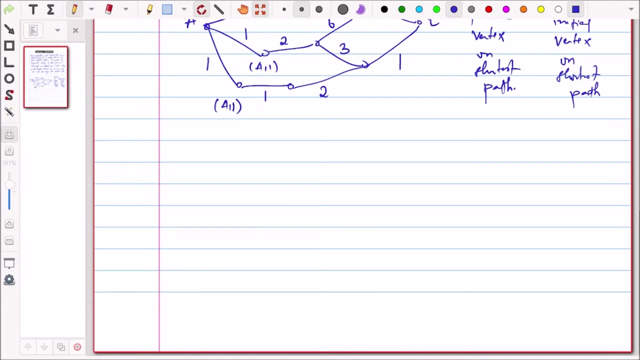 uh, so vertex. that's why they are calling it as e. okay, so let us call it as e. they are calling it as e another vertex e they are calling this n vertex a to e path, basically. so now let me give you the statement of the algorithm. 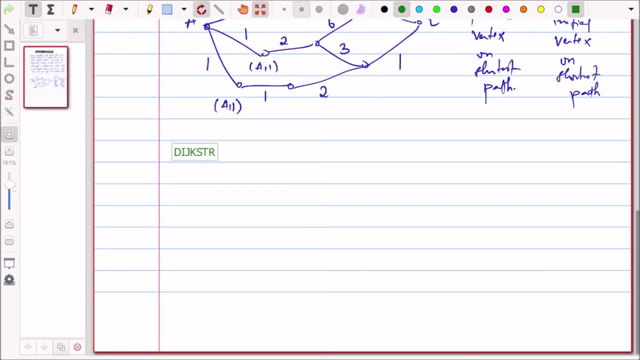 So there are just two steps. We will repeat these two steps again and again. So first step is: assign A label A, Because we don't have anything before A right Assign to A label. This is step one. 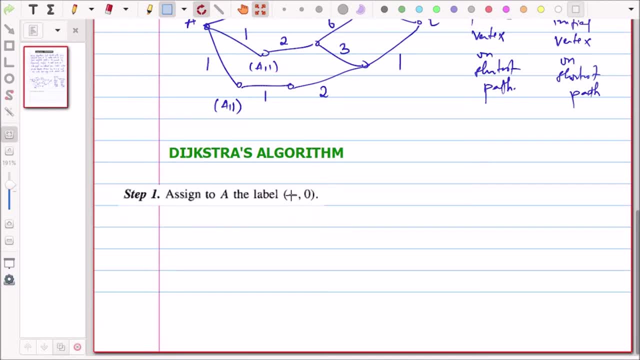 Assign to A the label minus zero. So this means dash, that is, there is no previous vertex to A. okay, And distance from A to A is zero, So it is zero, okay. That's why we are giving initial label. 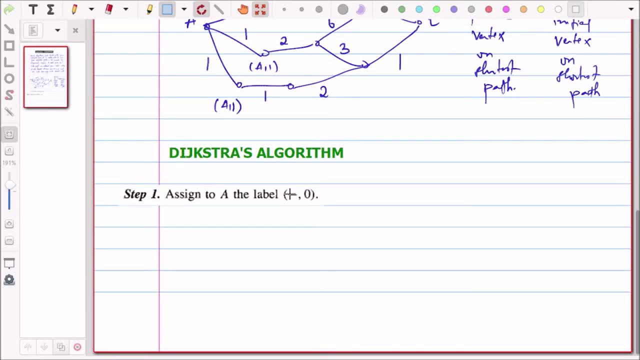 This is called initial label. okay, So initial label is dash, zero. Dash means there is nothing, And zero means distance from A to A is zero. So that's why we are giving zero label to A. Okay, is it fine? 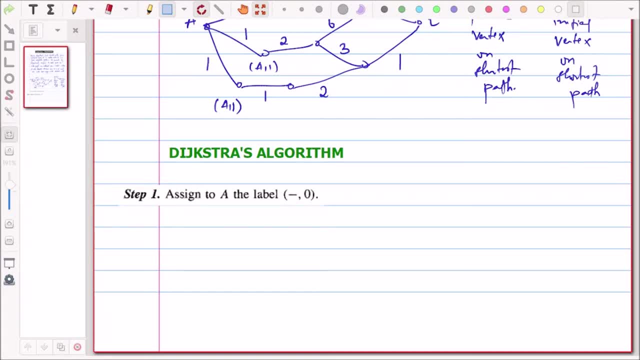 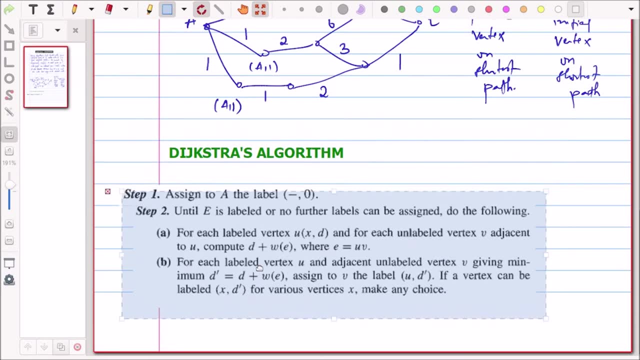 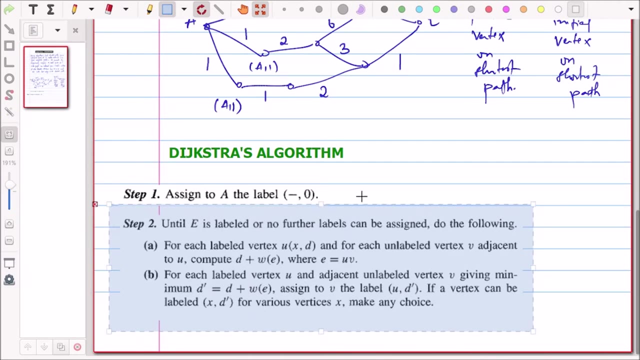 Yes, sir. And second step is: until we don't have A label, until we don't have E label, we will not stop and we will keep on giving labels. And how will we give the label For each labeled vertex? U, X, T. 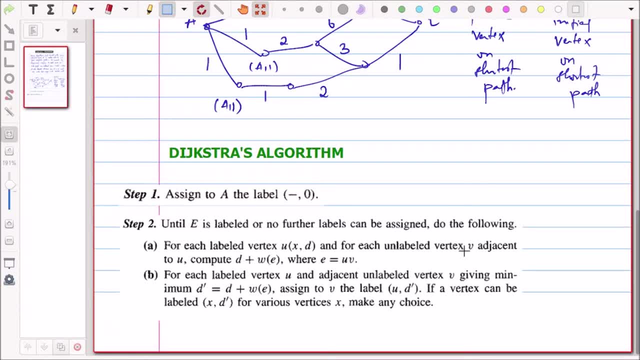 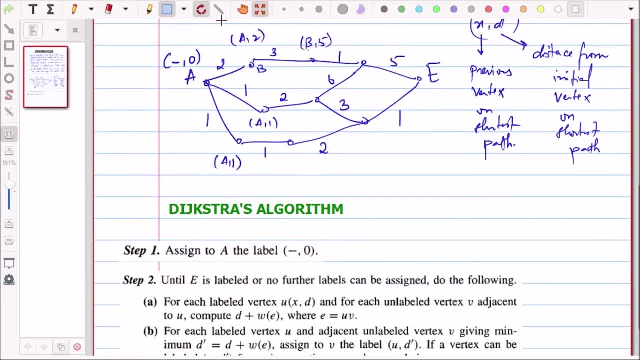 For any labeled vertex U, X, T And for each un-labeled vertex V adjacent to U. So all the un- Like we had a label here. we had labeled this, So we will see the adjacent vertex from this. 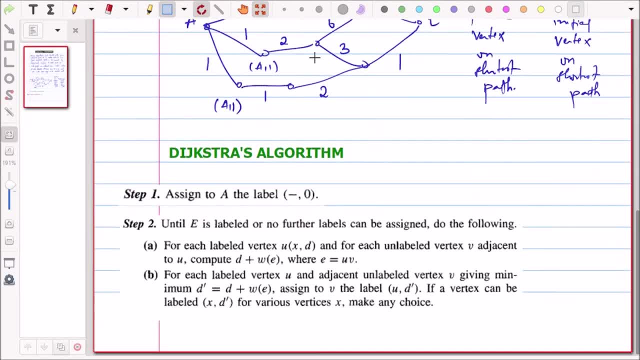 So this is adjacent, So we will label this. Okay, So what will we give to this? We will give this label D plus WE- D means the distance of this- And we will add its weight to it, Like we had here. its label was 2.. 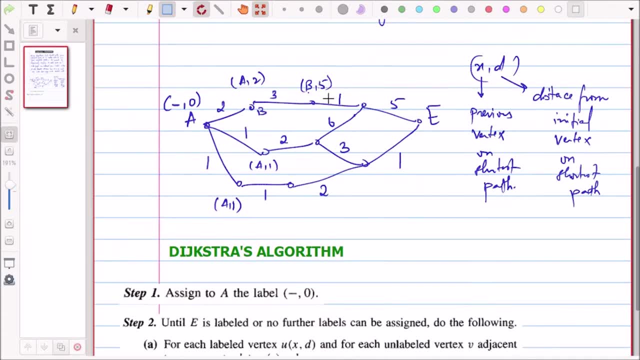 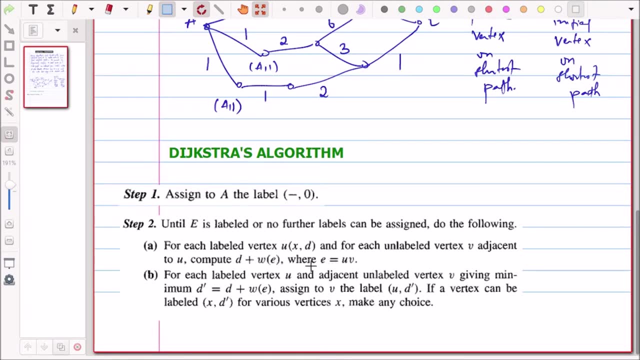 Then we added 3 to this, So we gave it 5.. Okay, And so D. our new distance will be this, D plus WE, And X will be the previous vertex. So U will come to it, Okay. 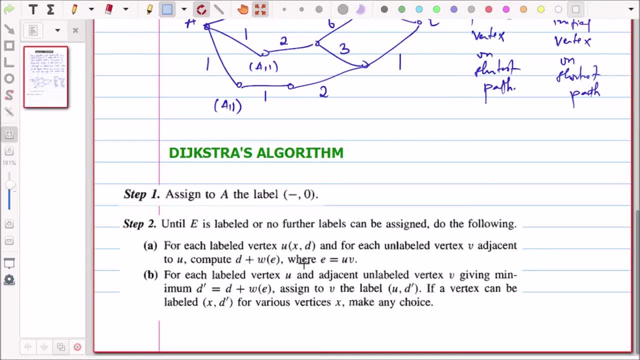 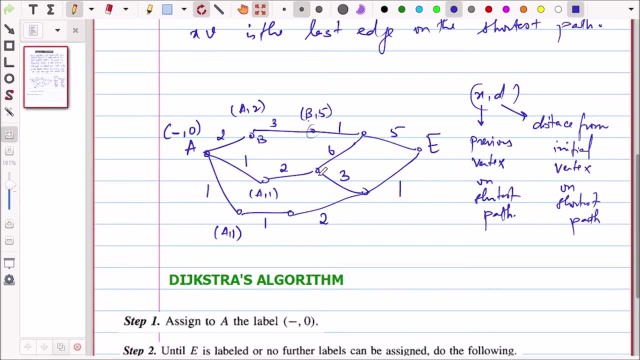 Is it fine. Now what will happen is there can be a possibility that if both of these were labeled, Okay, If we have this vertex and this vertex was labeled, So this is adjacent to this and this is adjacent to this. 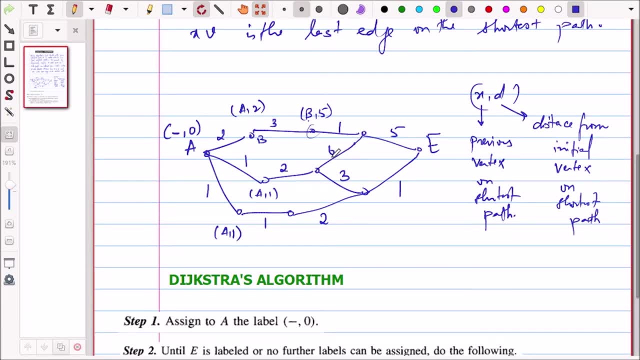 So the distance which will be less, we will give its label. We will consider that as the previous vertex. Okay, And if we see its label with this, then what will happen? This will be: if this is C, So this will be your. 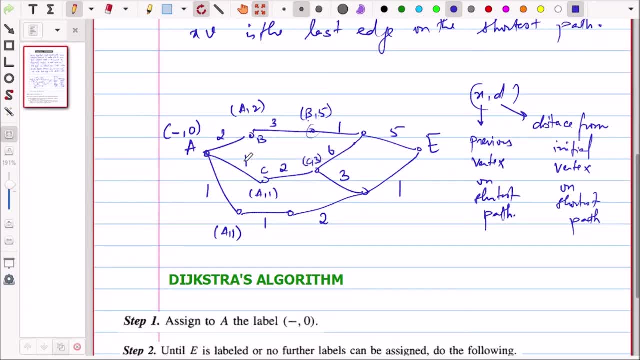 C and 3 will come right: 2 plus 1, 3 distance. So now its label. it has two labels. One is coming from this, one is coming from this. Now, what is the distance coming from this? 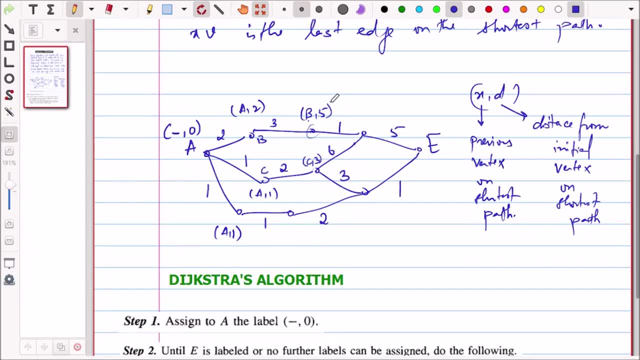 6 is coming. What is the distance coming from this? 6 plus 3, 9 is coming. So we will take this distance. We will take the 6th one. Okay, Yes, Yes, sir, Okay, now we will try. 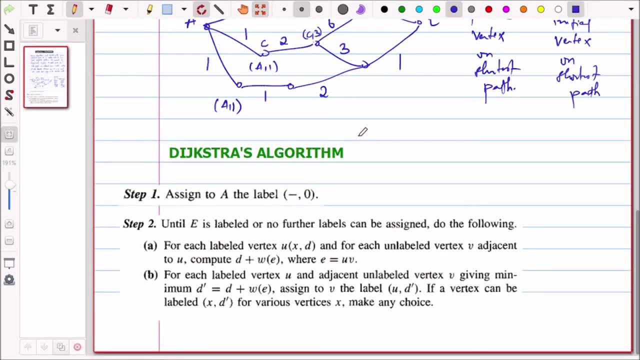 In this case it can be equal. Yes, it can be equal. So if it is equal, then you can take any one. See if a vertex can be labeled XD dash for various vertices, X. make any choice, it is up to you. 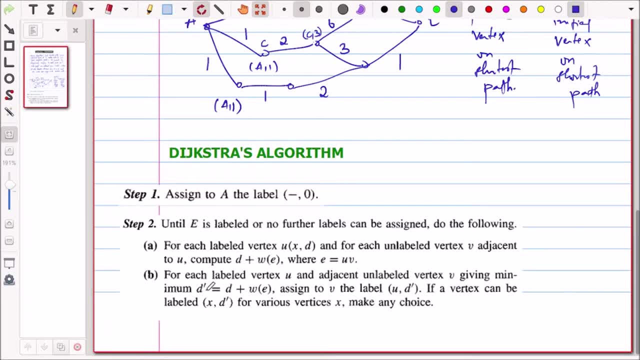 And here, what is it doing? first, Unlevel, giving minimum D dash, whatever the minimum D dash will be, first you have to give that label, but now, if it is coming equal, then you can give any label. that is your choice. 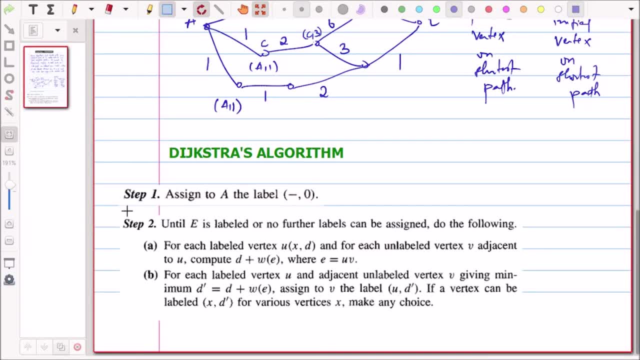 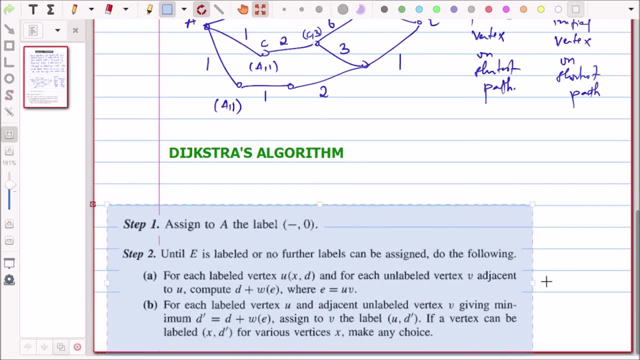 Because then it doesn't matter. if you take any path, then you are reaching at the same time same distance. okay, Then it's your choice. Which one is your choice? Same day, tolerate and Jam, And that's one, Or else you are patient. 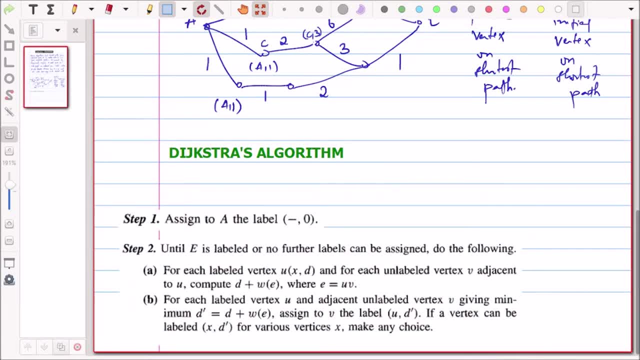 And then this may be a little out of sequence, that's me. I guess it is a little hard. I'll just say what is the way you want to see and hope not, So see. But if someone cannot make it that round, so we just go through it again and again same. 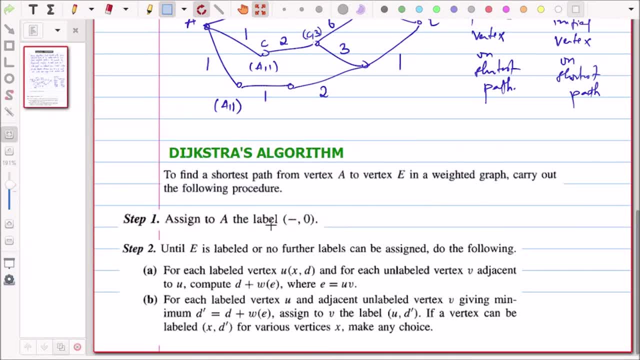 science. So it's easier. like this. You say it again and again: Pro 느�. I'm going to repeat it. I'm going to still repeat it, I'm going to write after it, I'm going to fashion不會. 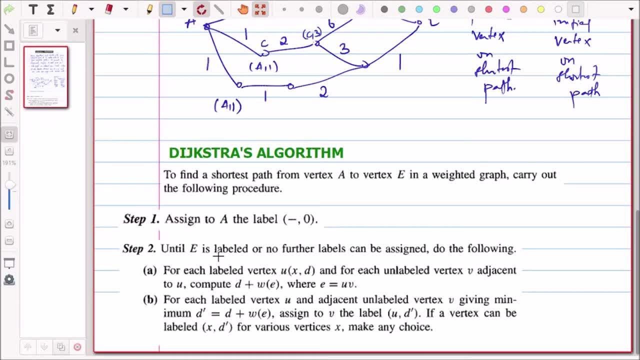 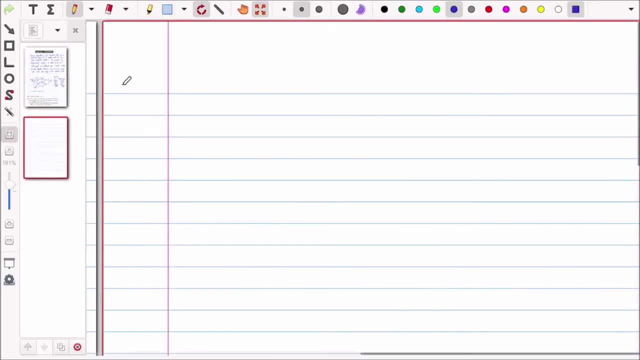 Okay, Uncle. what Didn't you tell me about? yes, is it clear? yes, sir, okay, yes, let us solve one question based on this. so we will solve this question using dexter algorithm. so question: find the shortest path between a and e in the following: 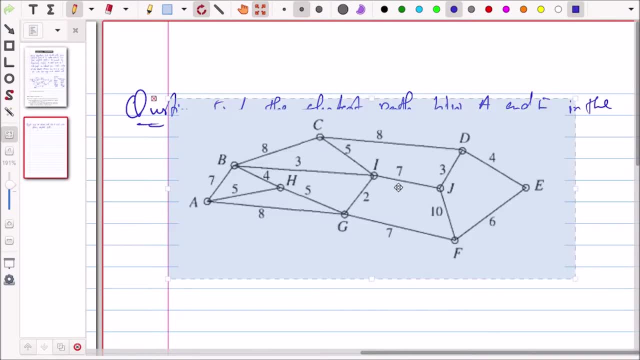 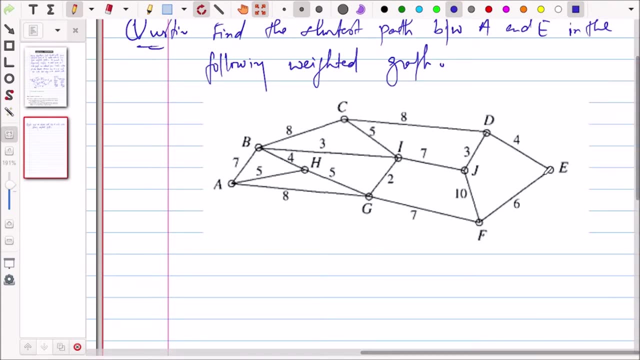 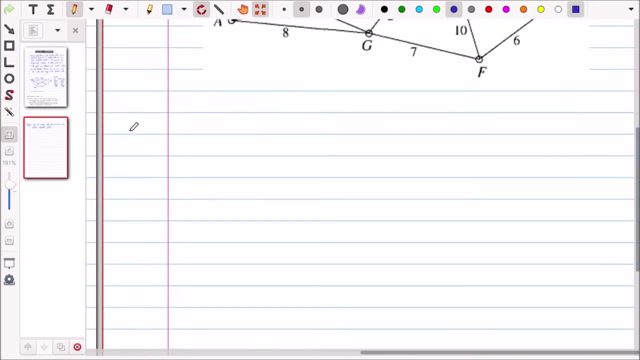 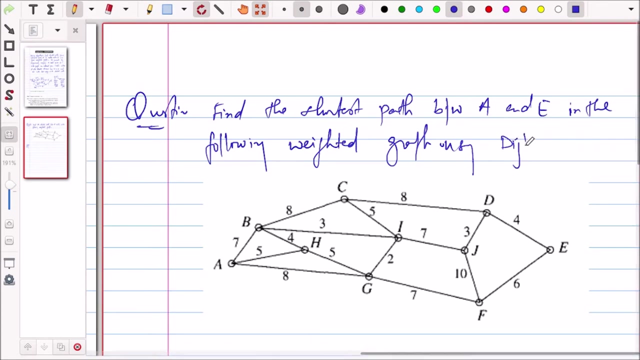 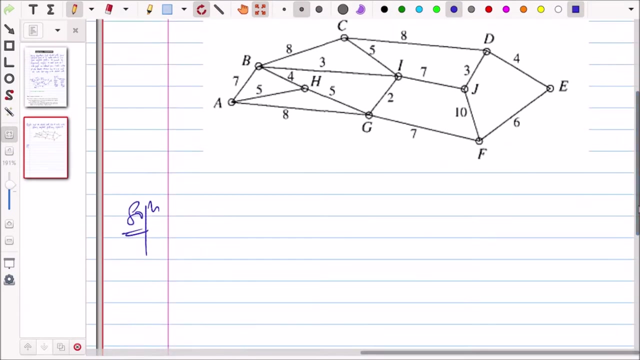 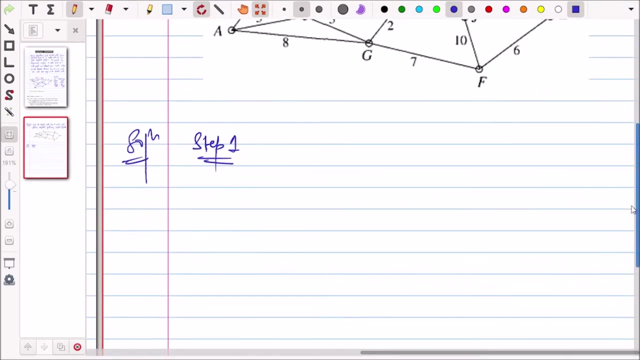 weighted graph. okay, so this is the weighted graph, so it's may have a. okay, is it clear? so let us start using dexter algorithm, using dexterous algorithm. okay, so what is the first step? step one: assigning a the label dash comma zero. yes, we will assign. 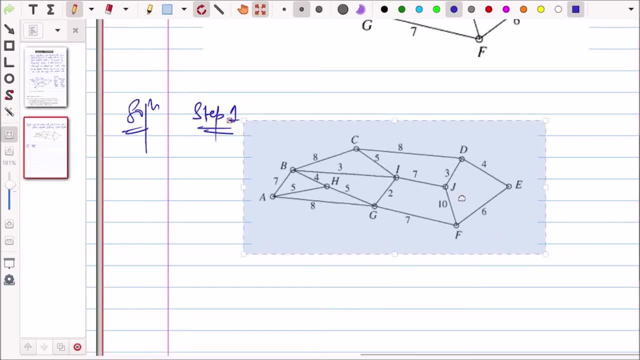 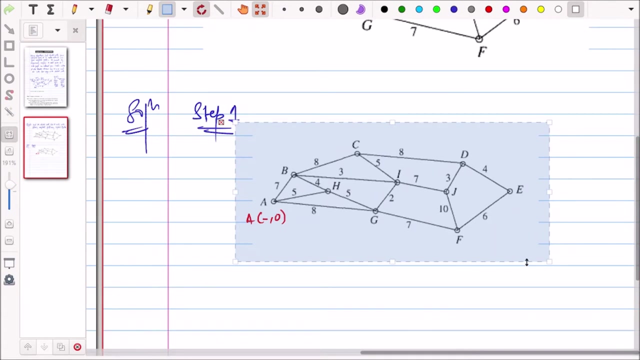 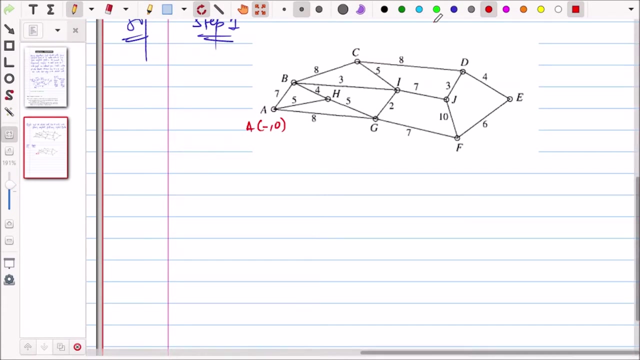 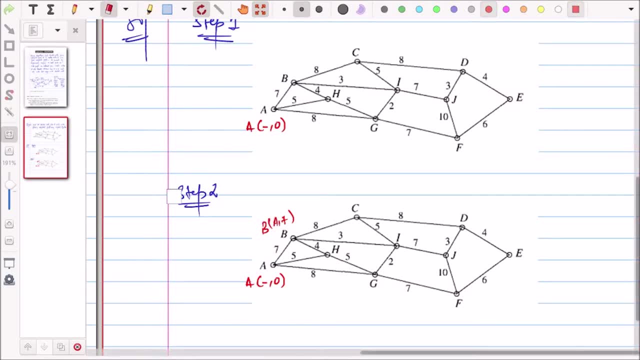 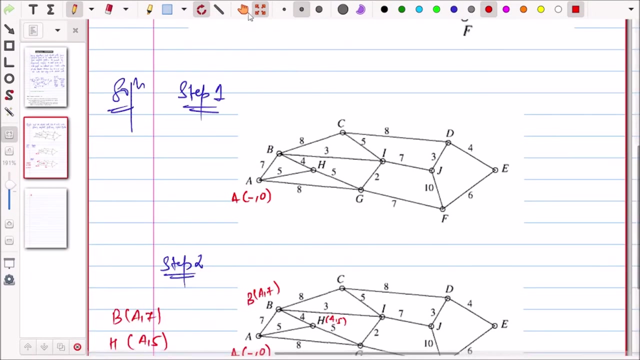 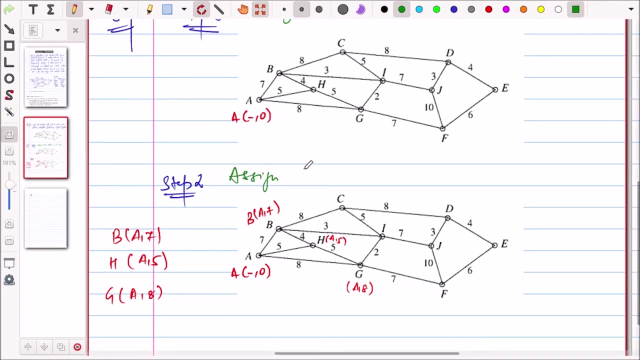 a comma five, so b is a comma seven, h is a comma five and g is eight comma five and g is a comma eight, zero plus eight, zero plus five, zero plus seven, so seven five and a comma eight, eight. right. so Jest Hm Linear Very Assign. label to unlabeled vertices adjacent to labeled vertex. 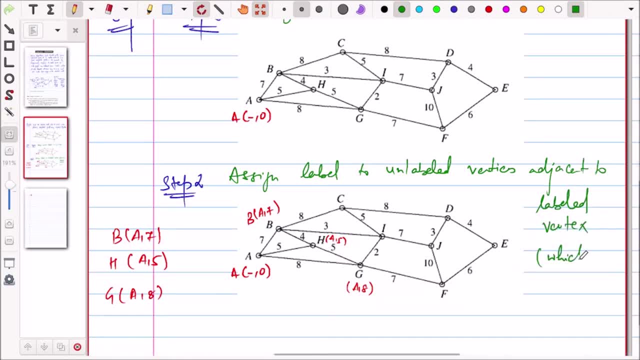 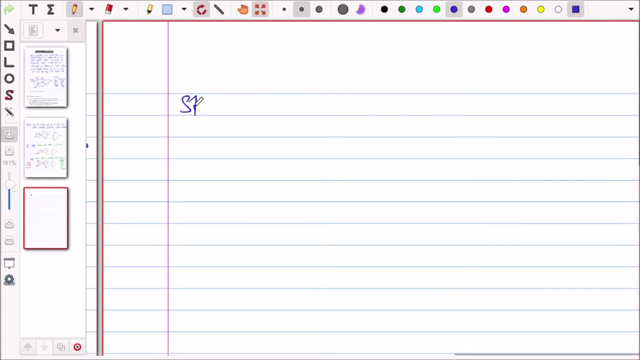 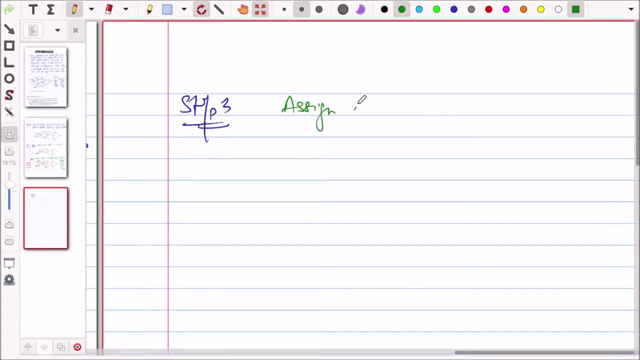 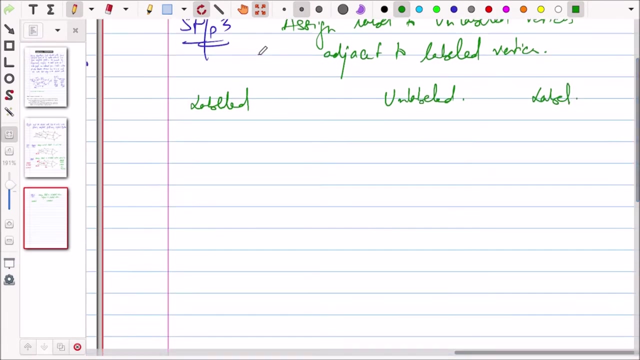 So again, we will assign Assign label to unlabeled vertices adjacent to labeled vertices. Okay, So in this case, which are unlabeled and which are adjacent to unlabeled, Let's make a table and give them a label. It is not necessary to do this in the exam, it is just for the understanding. 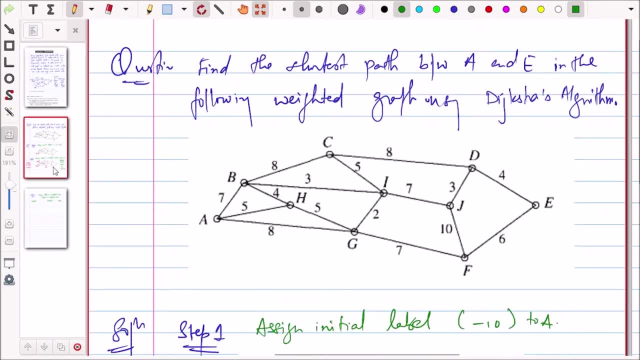 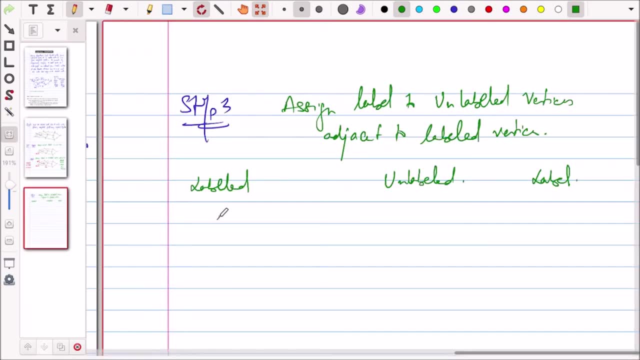 It is not necessary to do this in the exam. So what are the labels? we have? A, B, H, G, Because if you see this once, you will know for yourself A, B, H G, What is its label. 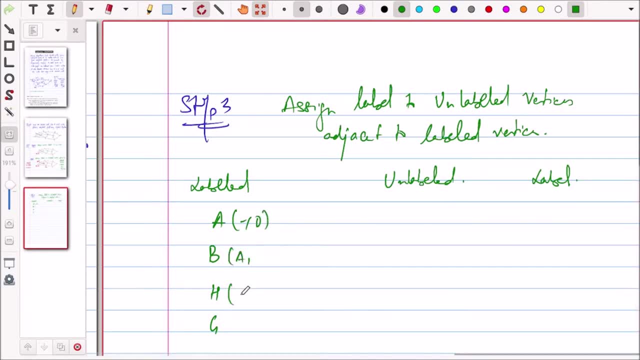 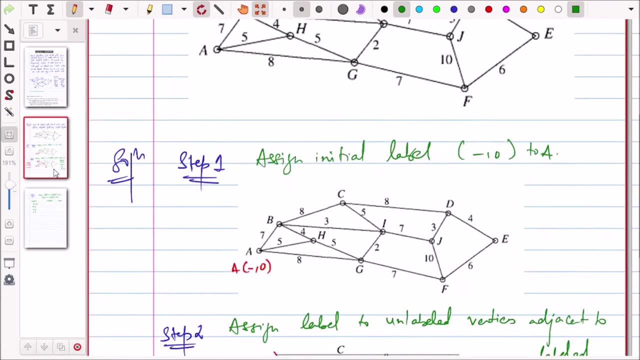 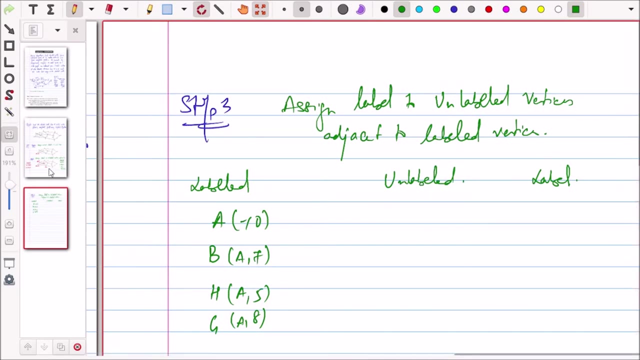 This is the label of A. This is the label of B. This is the label of A. What was A8?? A5, A7.. A5, A7.. Okay, now let me just copy paste this graph. We are making it so long to explain. 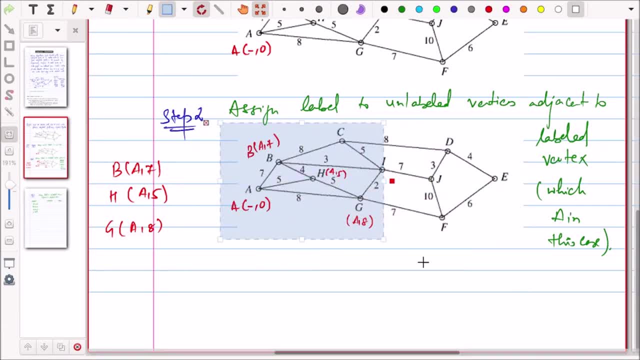 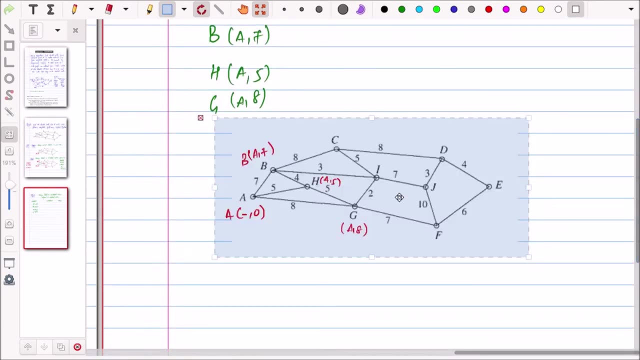 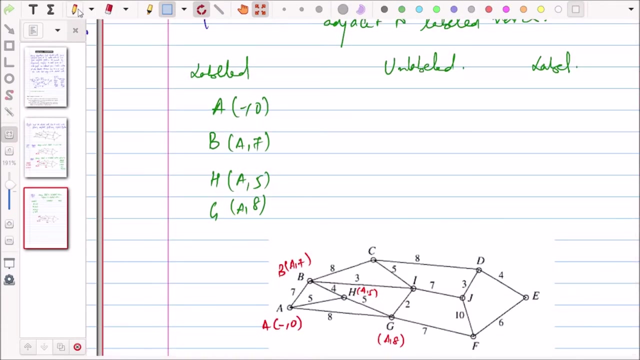 From next time, you can easily do it. There is no need to do this much from next time. So let's see how many unlabelled labels there are in A. There are no unlabelled labels in A right. Who are the unlabelled ones in B? 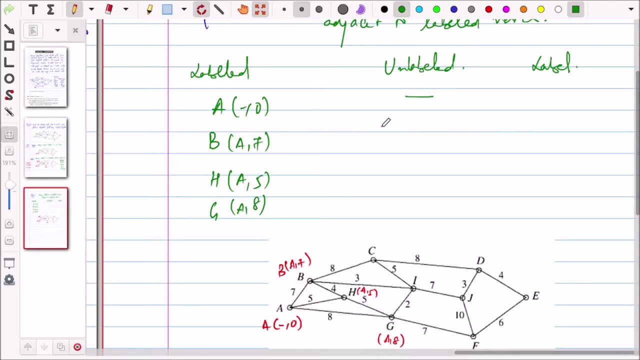 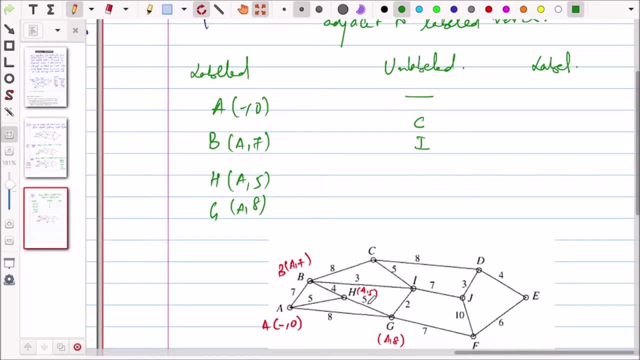 if you see what is the unlabeled of H, there is none right. but you can also change the label of adjacent vertices. if you have this less like 7 and this is 5 plus 4 is 9, so 7 is smaller. again, 5 plus 5 is 10 and 8 is smaller. 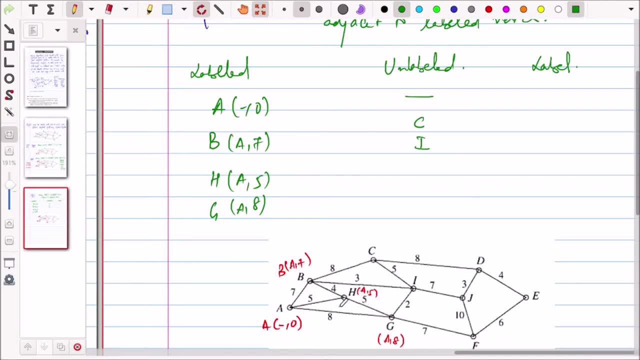 so you can leave it as it is. and 5 is same, so you have to check it. 8 plus 5 is 13 and there is none of H and G. is I? there is none of H, G is I and F? is it fine? yes, 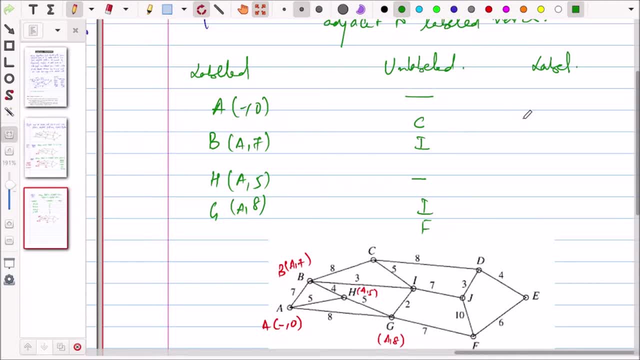 so what label will we give to C, B comma 15, yes, B comma 7 plus 8 is 15. and I, what label will we get from here? see, there are two labels of I, one is 7 plus 3 is 10, right, one is 10. 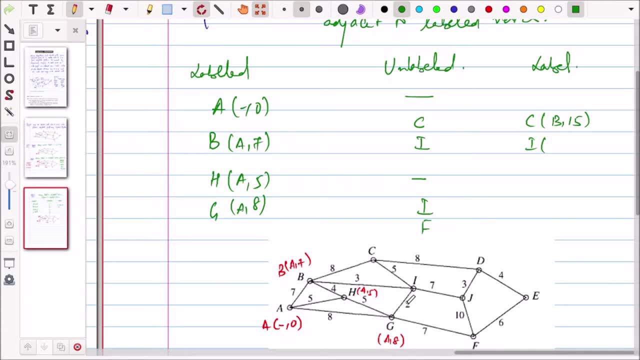 and one is 8 plus 2 is 10, so both are 10, right: 8 plus 2 is 10 and 7 plus 3 is 10. so you can give any one. so which one you would like to have, let's give G. 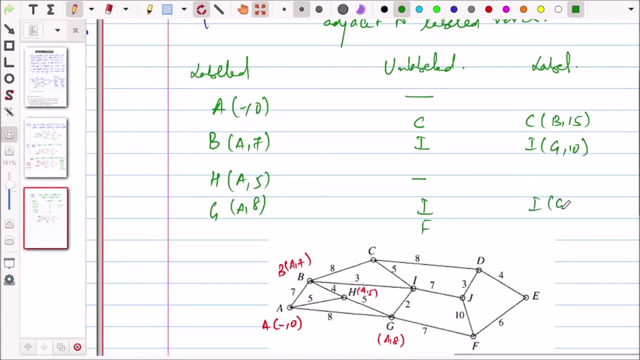 G is 10, so I here also. G is 10 and F is- or you can give it B10 once in this. ok, because this is for your understanding in the exam. you don't have to write this in the exam- and F is. let us label it as: 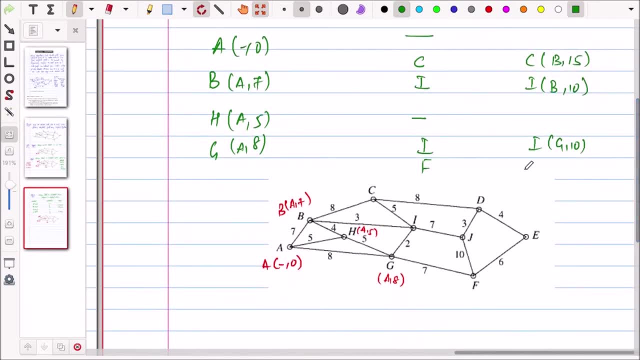 8 plus 7, G is 15, right? so now let us just give the label in graphs. so this will be G 15. this one will be- I will be- G 10, because 8 plus 2 is 10 and C will be B 15. 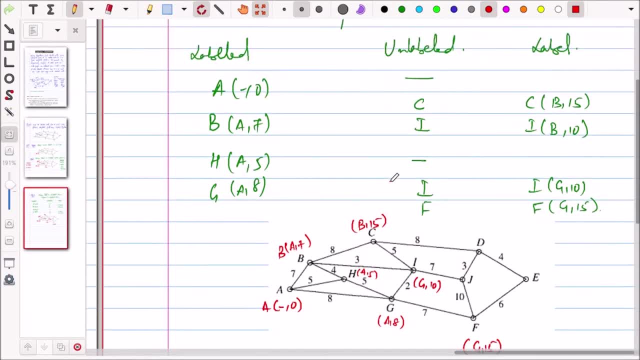 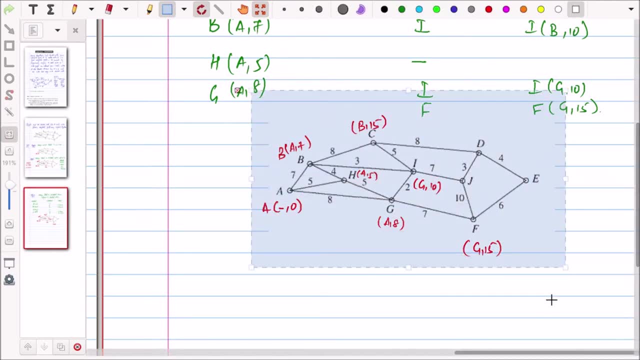 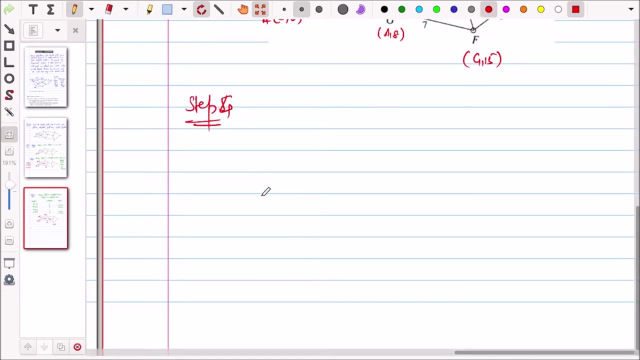 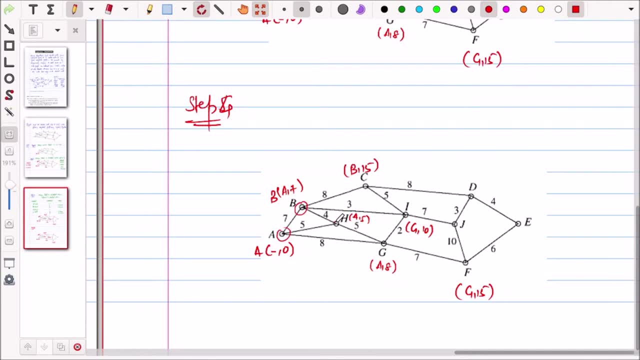 so this is already labeled: A is labeled, B is labeled, H is labeled, G is labeled, I is labeled, C is labeled, F is labeled. now we are left with this 3, so what level of E will come here? so what level of E will come here? what are the levels? 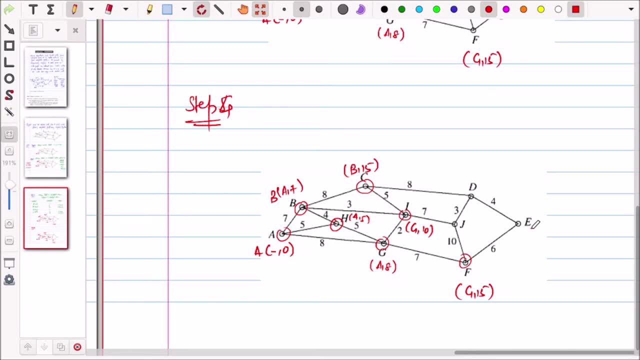 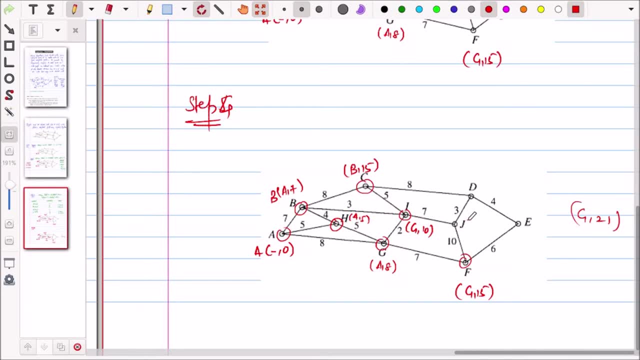 1, 1, 1, seven, seventeen, so you G 17 or a again. right, then for the 717, you get your head. do consent at this and this and this. this is the is B 23, but if you come from here then, sir, j equal to i, comma 17. okay, sorry, yes, i comma 17. 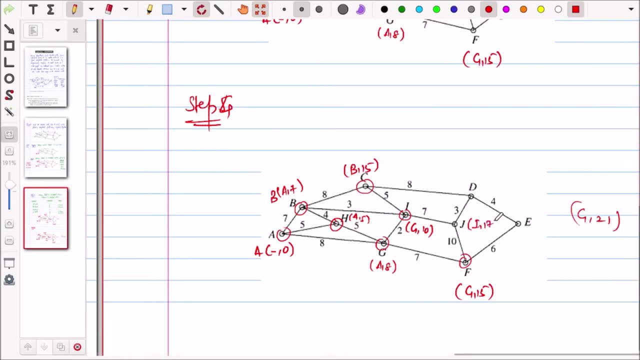 because it is coming from i, so i comma 17, right, and what will be the label of d? now look at the label of d if you liquid this: b comma 23 is there, but here what we have is j comma. b comma 23 is there, but here what we have is j comma. 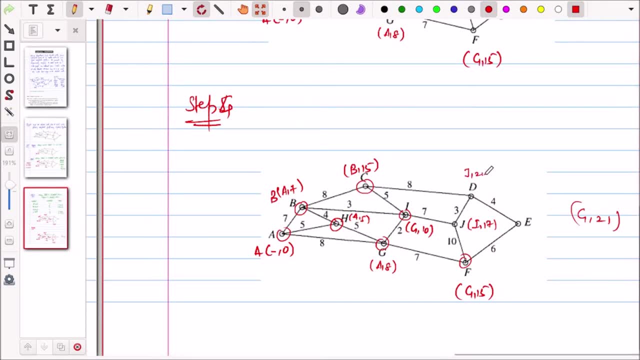 but here what we have is j comma, but here what we have is j comma 20, right, so we will put it as j comma 20, 20, right, so we will put it as j comma 20, 20, right, so we will put it as j comma 20. so. 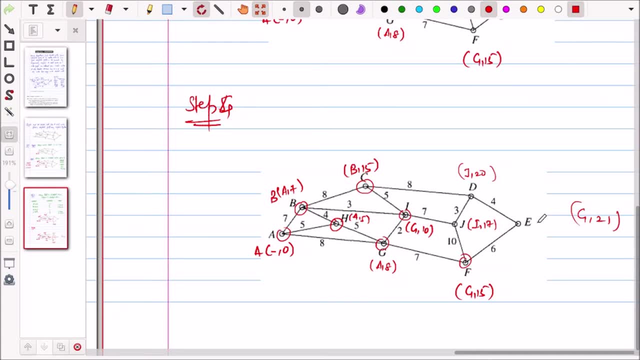 so so, 24, 24, 24, okay, okay, okay, or there's a 21. so this is the, or there's a 21, so this is the, or there's a 21. so this is the shortest. g21 is called because this is how you can label. 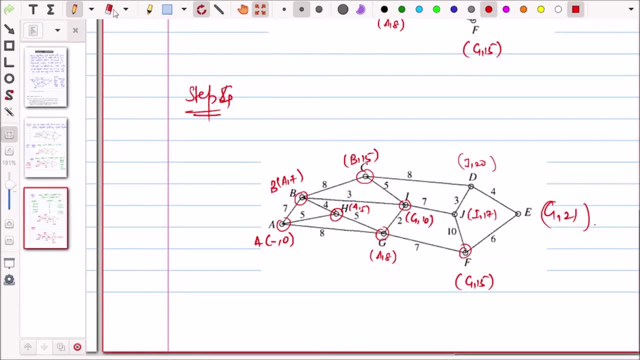 because this is how you can label, because this is how you can label: f comma 21, f comma 21, f comma 21, g sorry. f comma 20, sorry g sorry. f comma 20, sorry g sorry. f comma 20, sorry so f comma 21. 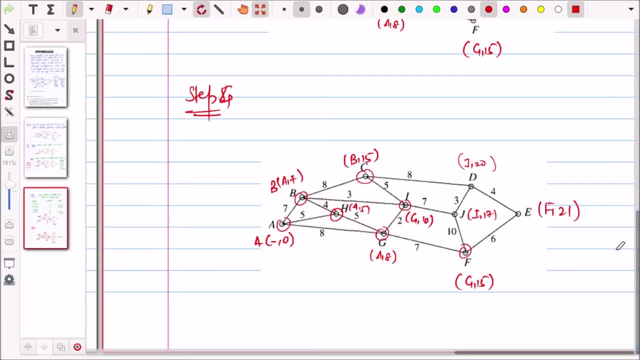 so f comma 21 g. sorry, f comma 21 g. sorry so f comma 21 g. sorry, f comma 21 g. sorry so now we just have to trace the path. so now we just have to trace the path. so now we just have to trace the path. we have to start with e and go to a. 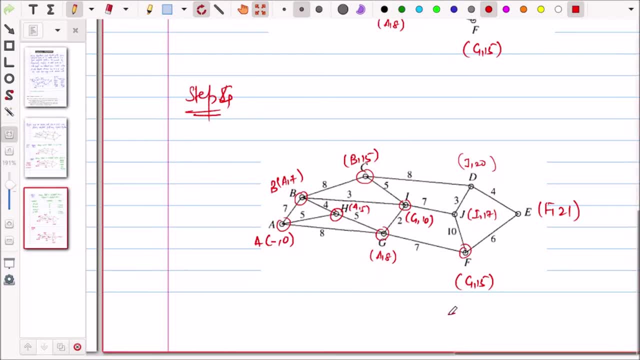 we have to start with e and go to a. we have to start with e and go to a previous vertex. so start with e, so e, previous vertex. so start with e, so e. previous vertex, so start with e, so e. then then then f, f, f, and what is the label of f? 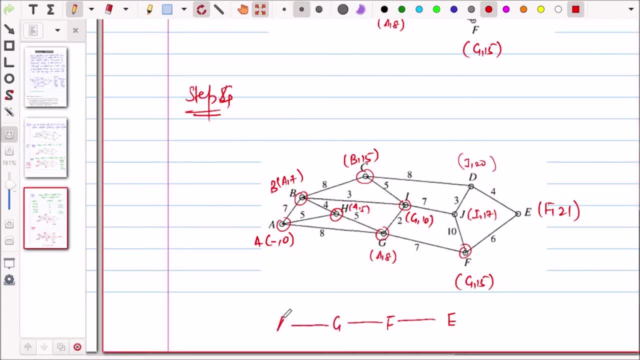 and what is the label of f and what is the label of f g and what is the label of g g and what is the label of g g and what is the label of g a. so this is eight a. so this is eight a. so this is eight, seven, six. so this is the shortest path. 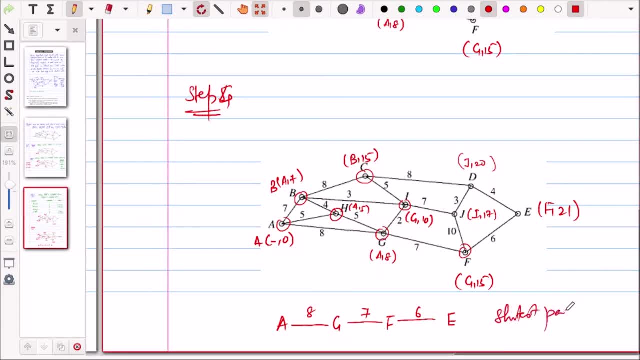 seven six, so this is the shortest path. seven six, so this is the shortest path from a to e, from a to e, from a to e. shortest path, shortest path, shortest path from, from from a to. is it clear? yes, sir, yes, so yeah, answer, if you look at this. 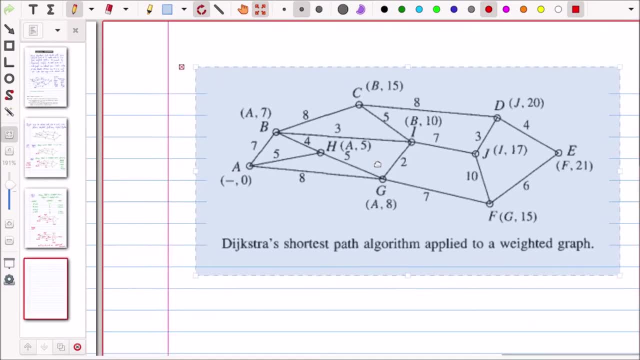 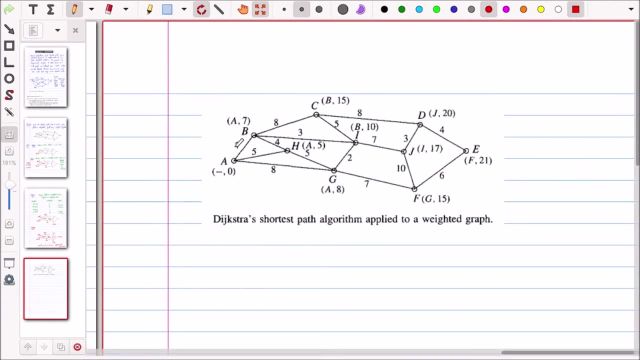 so yeah answer. if you look at this, so yeah answer. if you look at this answer, so almost similar answer. so almost similar answer. so almost similar, yeah, yeah, yeah, yeah, yeah. so if you look at this, so if you look at this, so if you look at this, so you started with initial this, then a7. 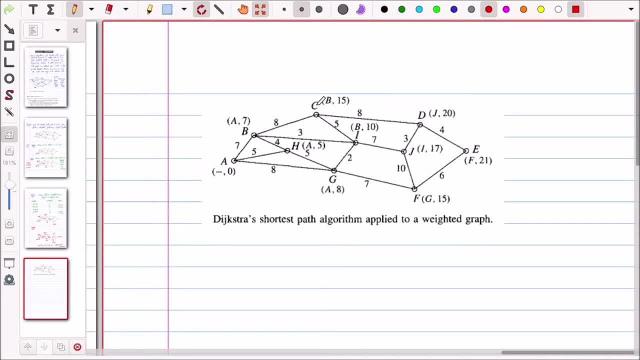 so you started with initial this, then a7. so you started with initial this, then a7, a5, a8. okay, then a5, a8. okay, then a5, a8. okay then. c is adjacent to this, so b15. c is adjacent to this, so b15. 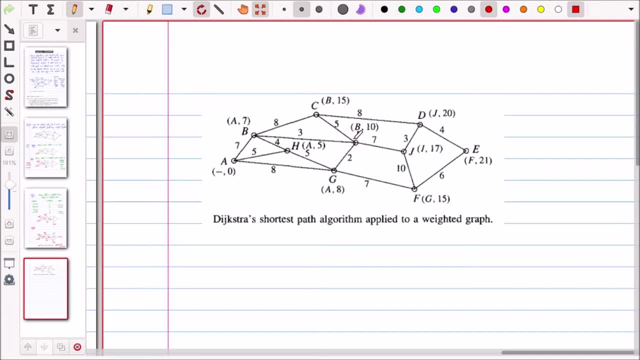 c is adjacent to this, so b15, or you are coming from b10, or you are coming from b10, or you are coming from b10 because it comes from this c. so it because it comes from this c, so it because it comes from this c, so it looks like b10 and this is a. 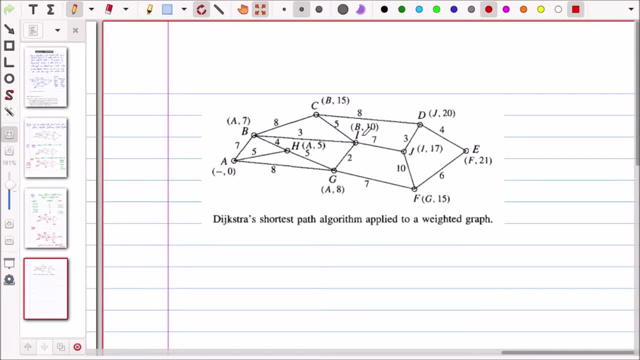 looks like b10 and this is a. looks like b10 and this is a job. neither again so f? g15 job. neither again so f? g15 job. neither again so f? g15 period. either say 10 plus 7- 17 period, either say 10 plus 7- 17. 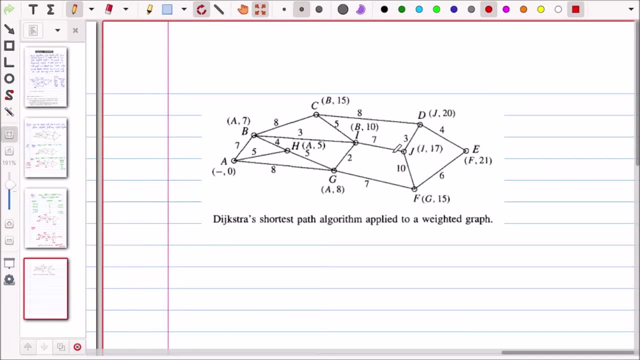 period. either say 10 plus 7, 17, because either say over the 25, because either say over the 25, because either say over the 25, so we will take this path. so i17. so we will take this path, so i17, so we will take this path, so i17. and then, yeah, say 15 plus 8 is 23, but and then yeah, say 15 plus 8 is 23, but and then yeah, say 15 plus 8 is 23, but he has a 17 plus 3 is 20, so we will. he has a 17 plus 3 is 20, so we will. 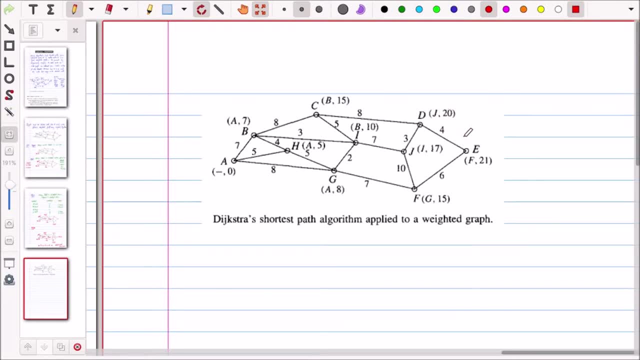 he has a 17 plus 3 is 20, so we will, we will label this as j20, okay, and then we will label this as j20- okay, and then we will label this as j20- okay, and then 20 plus 4 is 24, and. but here from here. 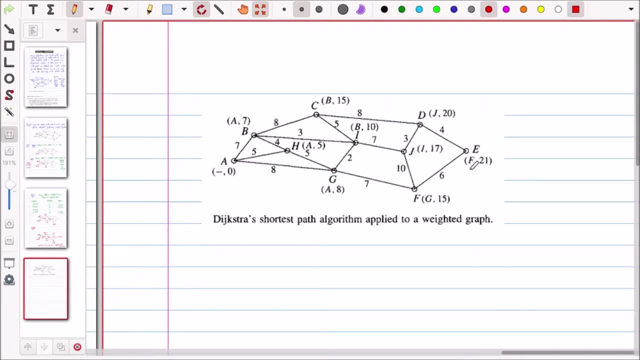 20 plus 4 is 24, and but here from here, 20 plus 4 is 24, and but here from here, 15 plus 6 is 21, so we label it as f21. 15 plus 6 is 21, so we label it as f21. 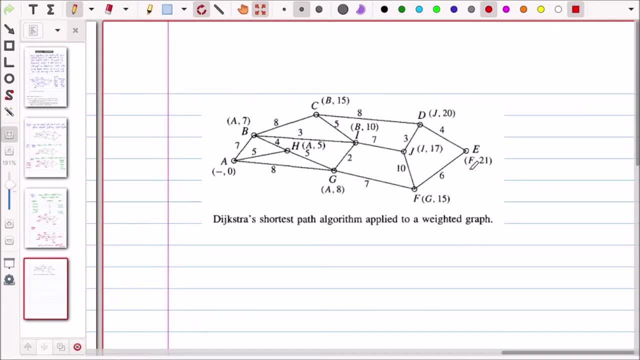 15 plus 6 is 21, so we label it as f21. so dexter's shortest path algorithm, so dexter's shortest path algorithm, so dexter's shortest path algorithm. applied to a weighted graph. applied to a weighted graph. applied to a weighted graph, because this is how you can label. 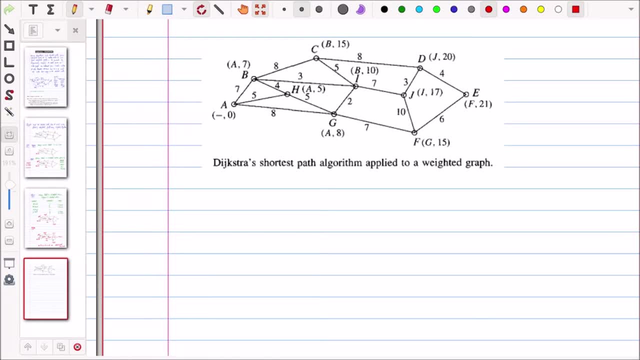 because this is how you can label, because this is how you can label, okay, okay, okay, is it fine? everyone this dexter's is it fine? everyone this dexter's is it fine? everyone this dexter's? algorithm, algorithm, algorithm, yes, yes, yes, okay, okay, okay. so a question. 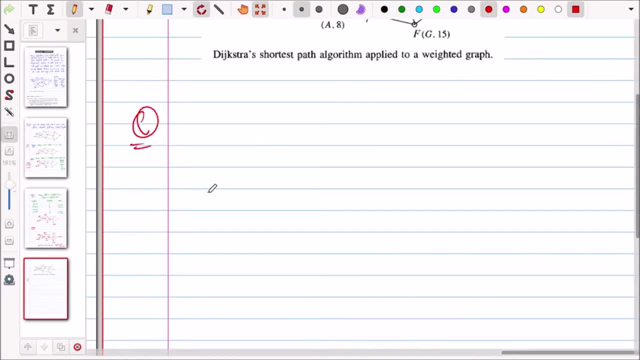 so let us do this question, so let us do this question, so let us do this question. okay, so direct the ring. okay, so direct the ring. okay, so direct the ring again, again, again. apply original version. there is one more. apply original version. there is one more: apply original version. there is one more version which we will do, so that's why it. 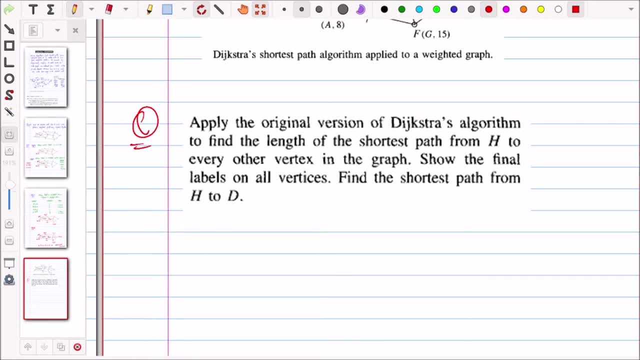 version, which we will do. so. that's why it version, which we will do, so that's why it is written. original version is written. original version is written. original version: okay, there is two versions of dexter. okay, there is two versions of dexter. okay, there is two versions of dexter algorithm. 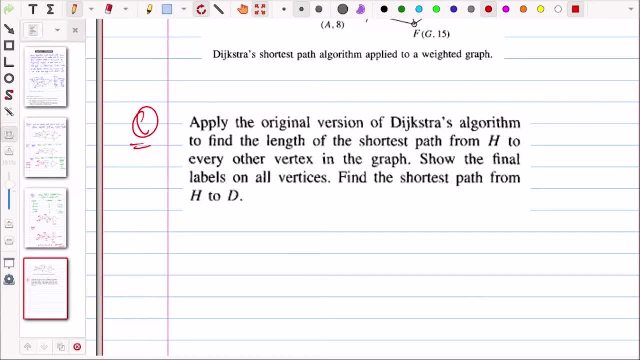 algorithm. algorithm. there is a improved version of dexter's. there is a improved version of dexter's. there is a improved version of dexter's algorithm and algorithm and algorithm and this, this, this, so improved version. maybe we will do so. improved version. maybe we will do. 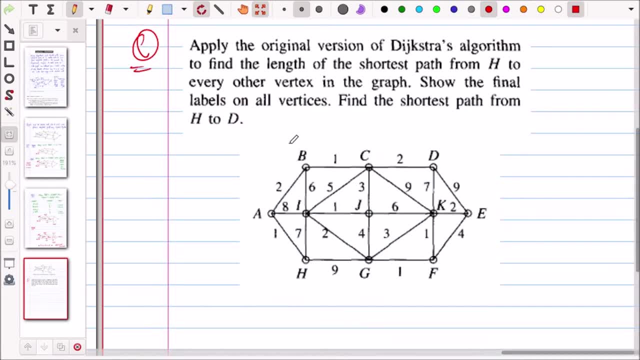 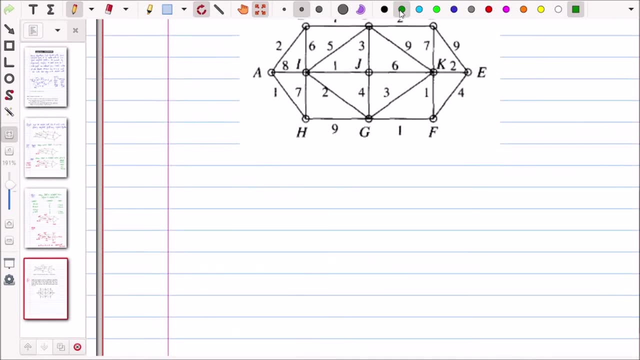 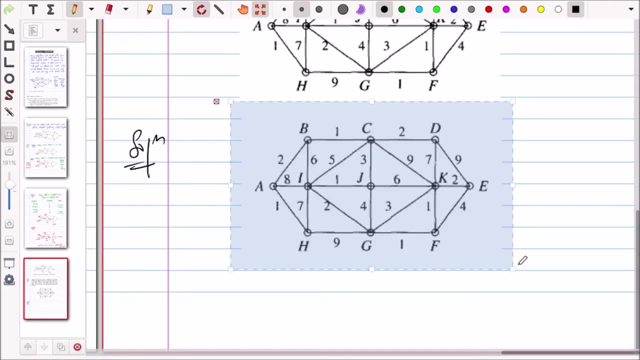 so improved version, maybe we will do tomorrow, tomorrow, tomorrow, okay, depending on the time, so let us. okay, depending on the time, so let us, okay, depending on the time, so let us. so let me just give make this diagram, so let me just give. make this diagram, so let me just give. make this diagram bigger, slightly bigger, so that we can. 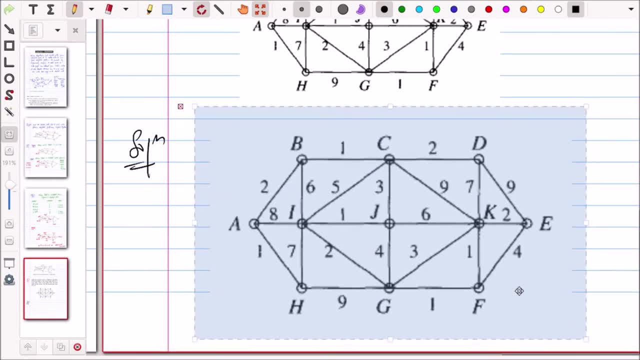 bigger, slightly bigger, so that we can bigger, slightly bigger so that we can label, label, label, okay, okay, okay. yes, let us start with. so we have to start. yes, let us start with. so we have to start. yes, let us start with. so we have to start with h and we have to reach d. 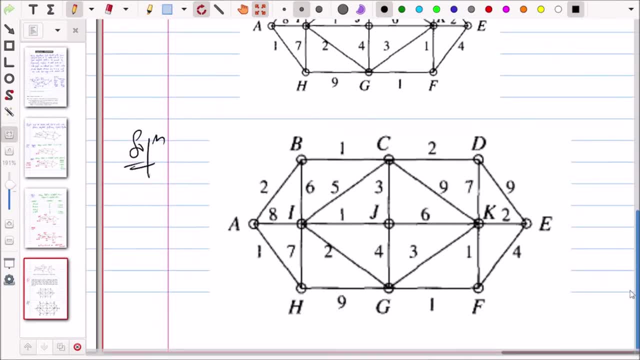 with h and we have to reach d with h and we have to reach d. so d is our final vertex and h is our. so d is our final vertex and h is our. so d is our final vertex and h is our initial vertex. so h could label then. 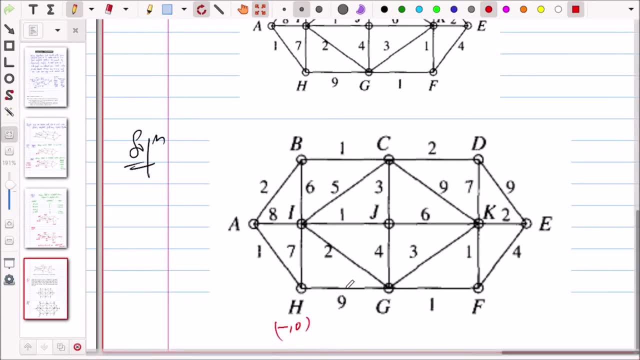 initial vertex, so h could label. then initial vertex, so h could label. then let us give the label, so it will be. let us give the label, so it will be. let us give the label, so it will be: zero right, zero right, zero right. i'm neighboring vertex. 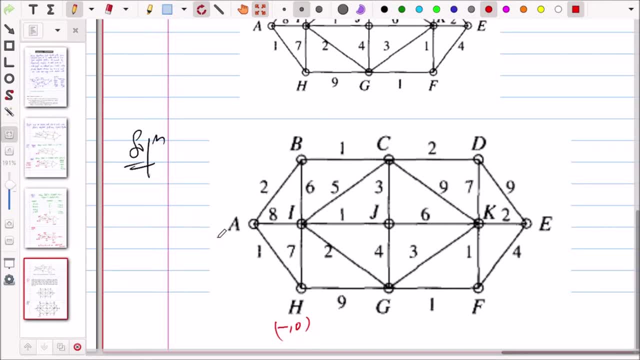 yes, yes, yes. so what will be the label of a or h comma one, h comma one, what will be? or h comma one, h comma one? what will be? or h comma one, h comma one, h comma one? what will be label of g? what will be label of g? 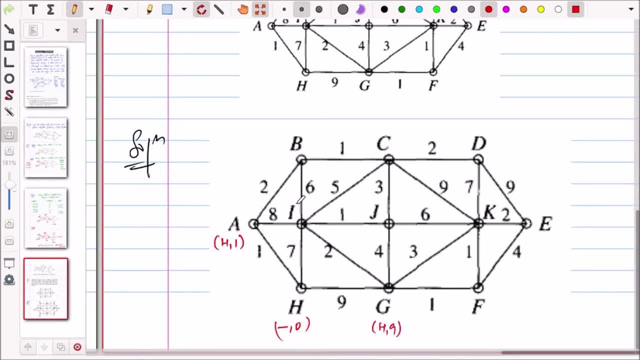 what will be label of g, h comma nine? what will be label of i? yes, i can even cover. yes, i can even cover. yes, i can even cover h comma seven, if there are any other vertex, h comma seven, if there are any other vertex, h comma seven if there are any other vertex. so three vertex are the same. so we have. 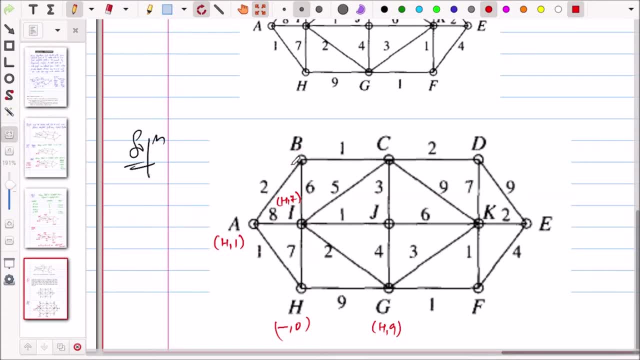 so three vertex are the same. so we have. so three vertex are the same. so we have. given three labels, now come to b. given three labels, now come to b. given three labels, now come to b. so up next, unlabeled concept b. so up next: unlabeled concept b. 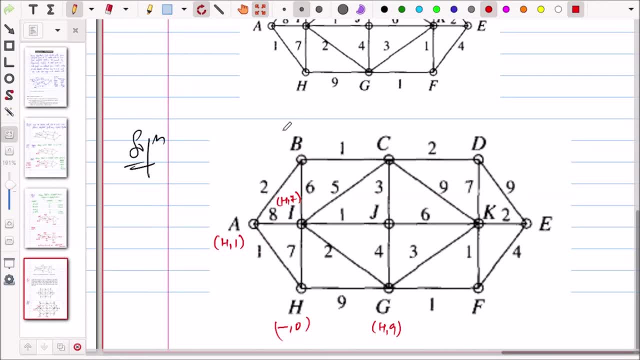 so up. next, unlabeled concept b: what is the label of b? what is the label of b? what is the label of b? two plus one, three, so a three from here. two plus one three, so a three from here. two plus one three, so a three from here. seven plus six. 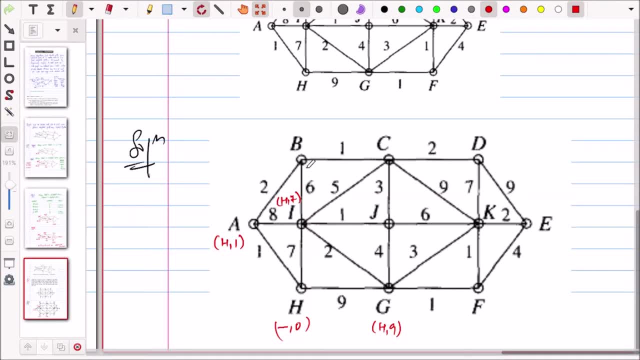 seven plus six. seven plus six, thirteen, thirteen, thirteen, right right right. seven plus six, thirteen. seven plus six, thirteen. so this is not from here, and which one is so this is not from here, and which one is. so this is not from here and which one is yes. 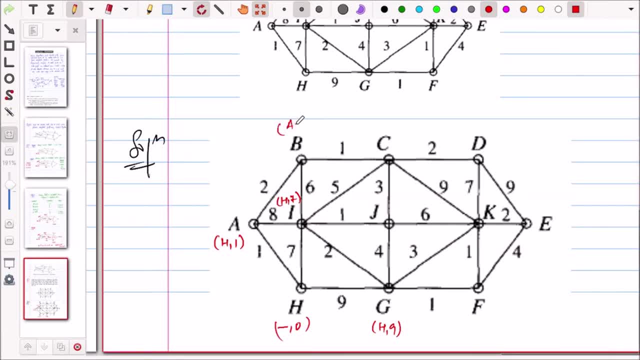 yes, yes. so the a is this, b is so the a is this b is so the a is this: b is a comma three, a comma three, a comma three, and what will be the label of j and what will be the label of j and what will be the label of j here? 9 plus 4, 13. 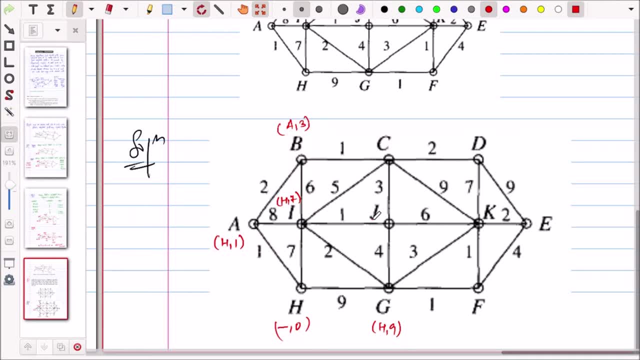 here: 9 plus 4, 13. here 9 plus 4, 13, so we won't take this from here. we have, so we won't take this from here. we have, so we won't take this from here. we have seven plus one eight coming. 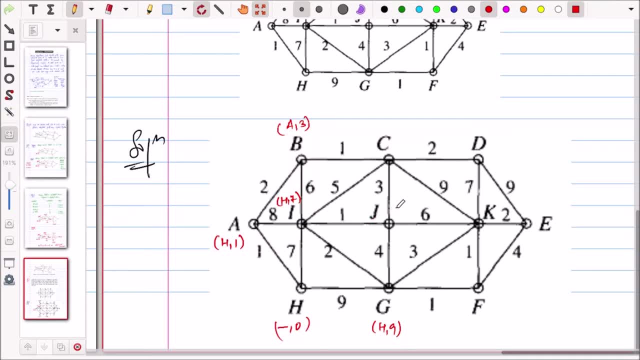 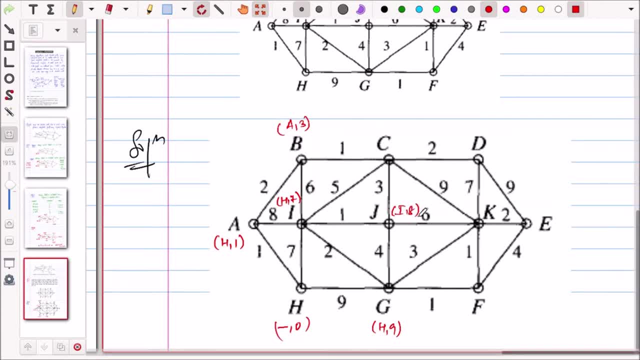 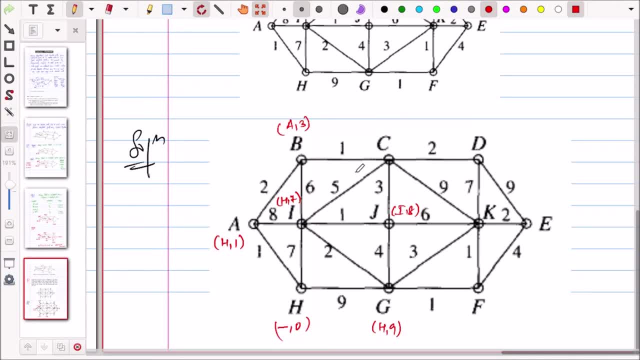 able to go there, go see scale able may have a scale centenar I can send to see. can able to go there? go you can see is saleable up now. come either be for either. so let us label it as before: ticket right, is it right? yes, up, consider this. yes. so this is before. yes, yes, F will be. 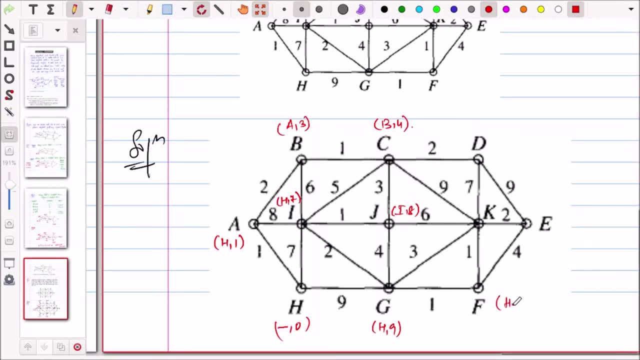 yes, F will be, yes, F will be F for an extension, even be today and so after here, next, and then K, k, k, push it resist 14, Hi, 4 plus 9, 13 high, or USA, 10 plus 1, 11, Or is there say 9 plus 312?? 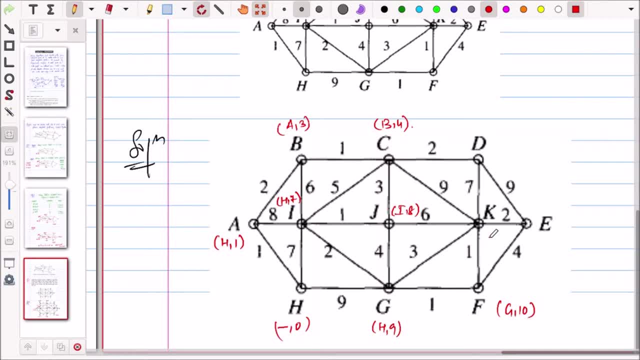 So, concerning you, Ask for my lover, Yes F, Mama, 11.. OK, or even in our pass, yoga K F Our purpose. We have labeled this, We have labeled this, We have labeled this Label, this label, this label, this. 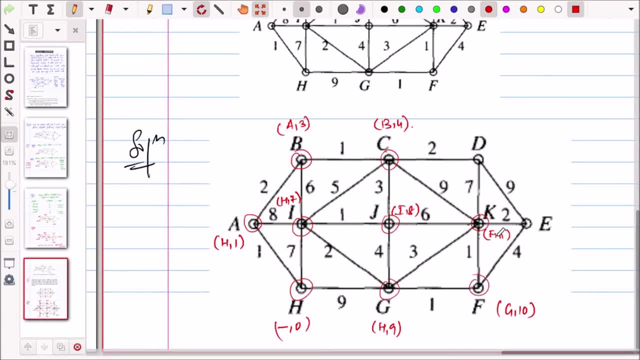 And label this also. No possibilities: 11 plus 2.. 30 or 10 plus 414.. Take it. so what we will take, Lady, is also like K13, right, And this is your C6.. Take it Here's: 4 plus 2, 6.. 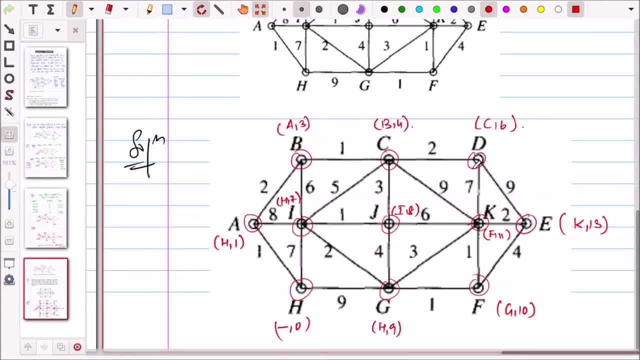 So sorry. level of help: Yes, Shortest path is so you start with the. So shortest path is D, D, C by, D, C by- This is me- And then C to be, to be co-labeled S car And then be too. 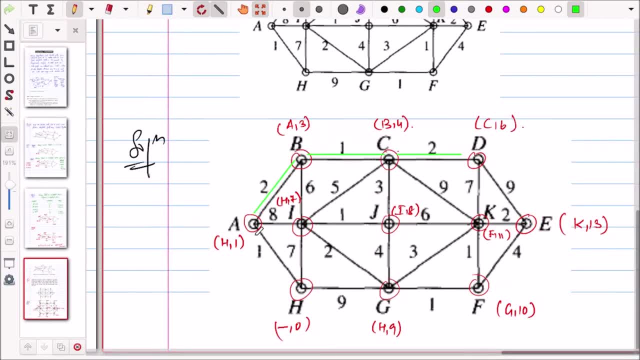 He will be I as, And then. So this is our previous word, It's for you, these are. you have. It says baby based basic, that your previous. They say: if I die, label Saatma, if we can trace back, okay, yes, so you can write it here. 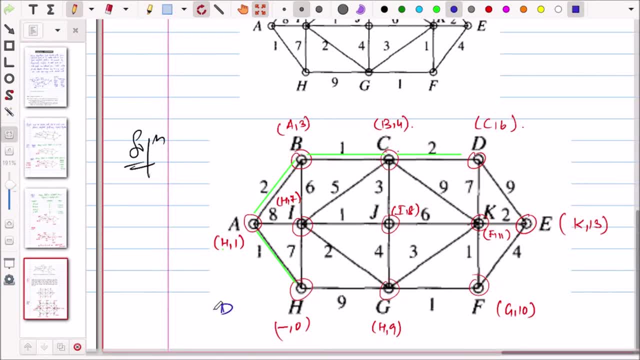 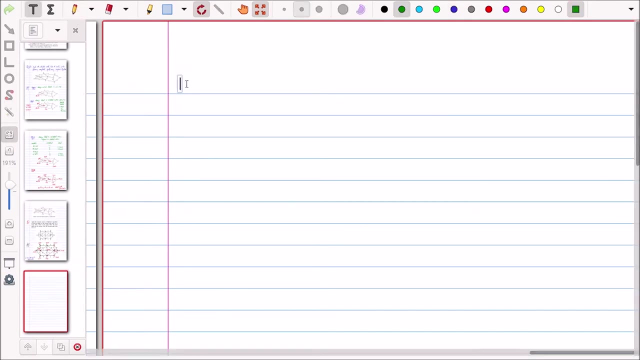 so d, d, then c, then b, then a, then h, shortest path. okay, is it fine? is it fine pieces? okay, now let us do improved dexter's algorithm. what is there in this improved extra algorithm? so why it is called improve? because it's polynomial. this is uh. its complexity is, it is of. 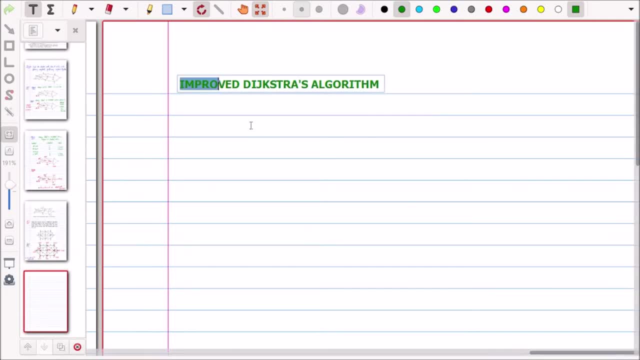 order i'm. i have told you already it is of order. this is of order n square, okay, so this can be solved faster. this is right. so that's why it is called improved extras algorithm. so there is slight improvement in this. so let me just give you the steps so you'll understand. 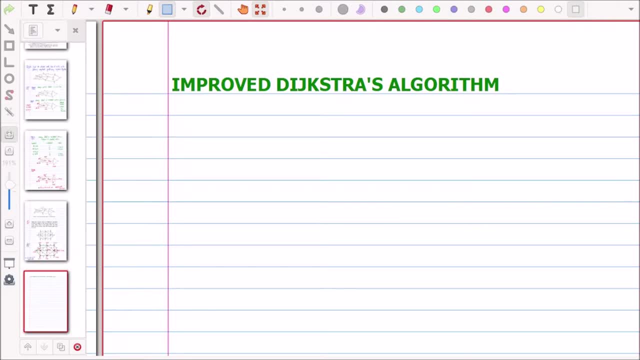 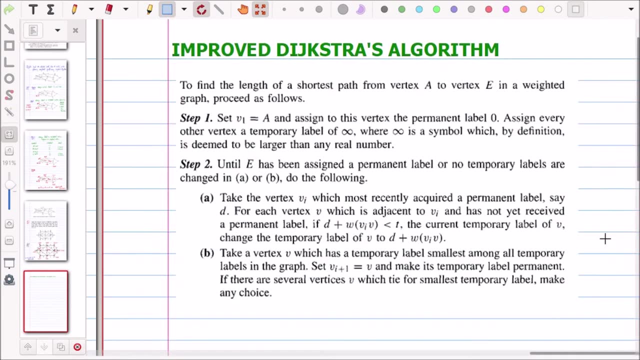 the steps and then we will apply it in the same example that we did earlier. so so what we do is: so we have to find shortest path from a to vertex c in a weighted graph. so what we do is: step one is we assign to this vertex the permanent level zero, so initial vertex. 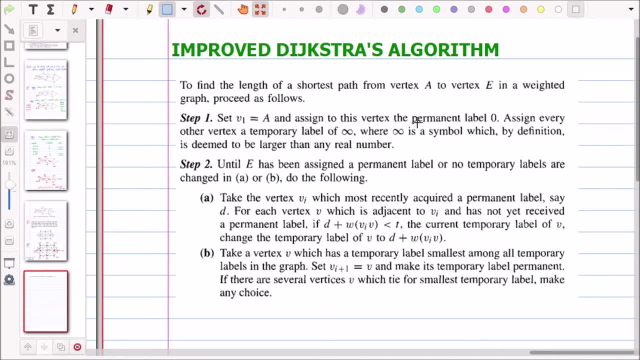 say so, permanent level: zero and every other vertex will have temporary label infinity ticket. so first step may. first, vertex label is zero and every vertex has temporary label: infinity. infinity seem to be a very large number, so we can. we are giving this infinity to other numbers, is it fine? 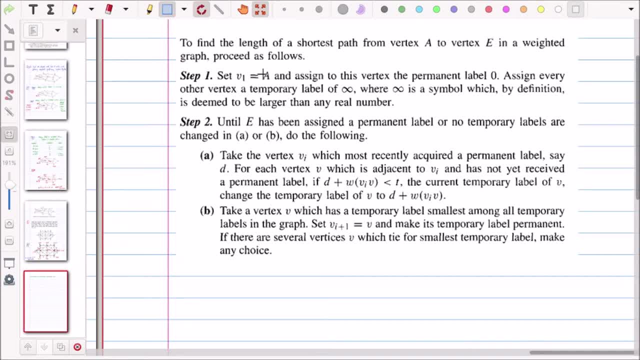 okay, now what will happen is first: so echo, zero level lady, so %HESITATION. so so they are first in the first step. they are at distance infinity from a. now what is the next step? here i mean next step, repeat: 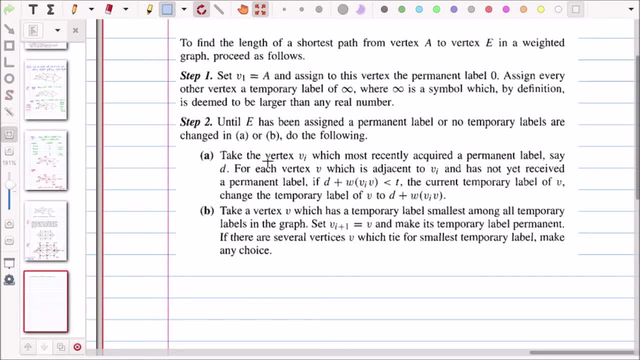 which most recently acquired our permanent level, just cause, of say, recent. may permanent label me like ticket. the first step make it a component level, the. I thought our VI will be one, would I camera or us, for each vertex V, which is insane to me, I and has not yet received a permanent label. what we will. 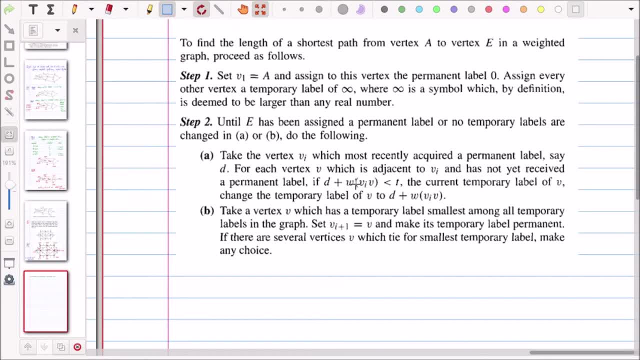 give. we will give if D plus W. so, Joe, we wait over VI. Vika was for added. okay, I'm just gonna enable. the thing is that current temporary level of V ticket. so basically, let me just show you or us go on a label. the thing is your distance. 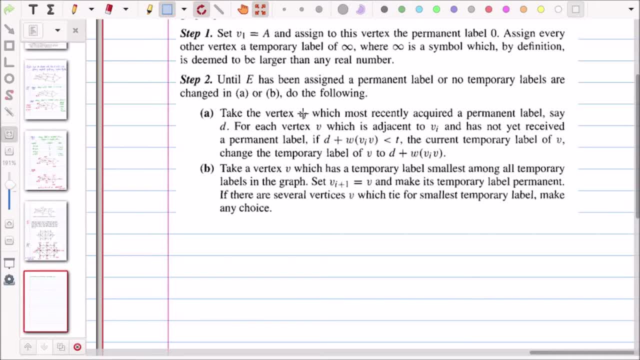 was distance, like a day ticket of bees, just a be one the other than the level ticket. our next level is adjacent. I'm us go V to us equal dengue. discuss up second level over Bucky. what Bucky core hum labor nahi dengue. 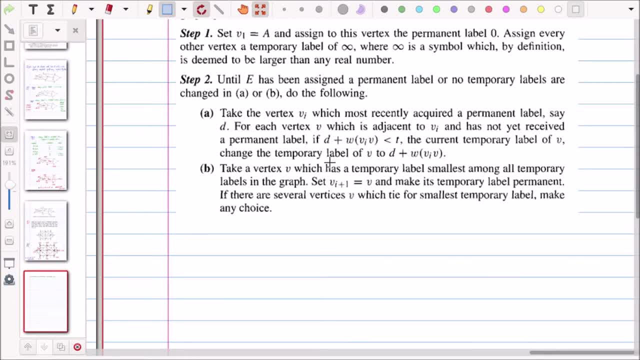 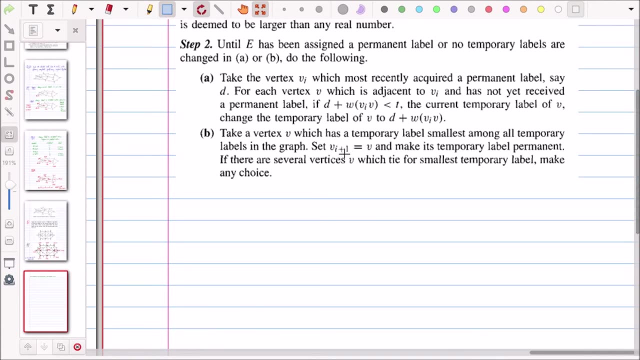 some material. I must see what extra level dengue just got label. come over subseminum, allow a sequel, a building a or kissy-koo label. he didn't give us eco. we will call it as V to take a set VI plus 1 equal to V and make it. 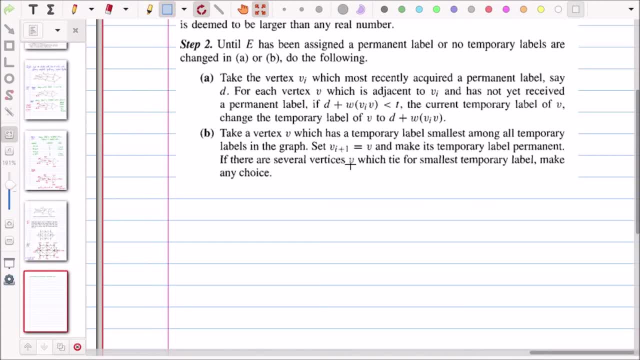 separate label, permanent, and if there are several with vertices V which tie for smallest temporary, temporary, they will. we can make any choice ticket. so let us just see this in the example, then you will understand this. okay, so let us just see this. so let me just give you the same graph. let us take 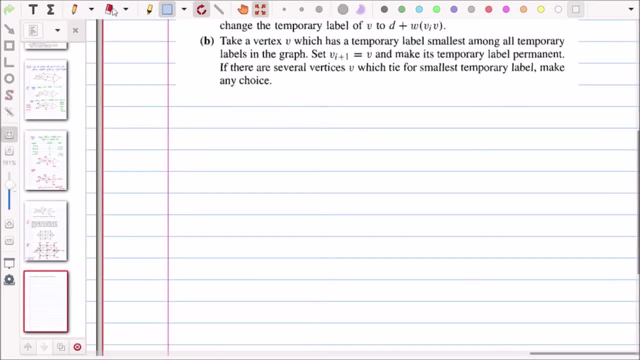 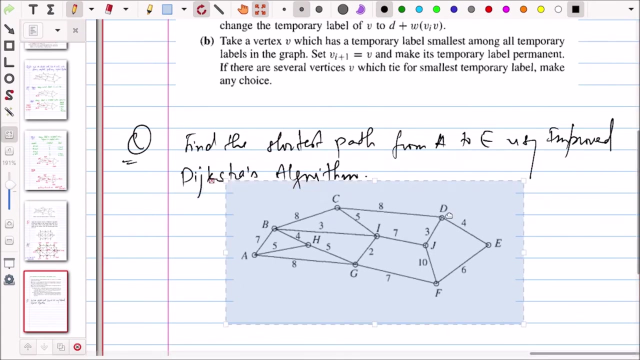 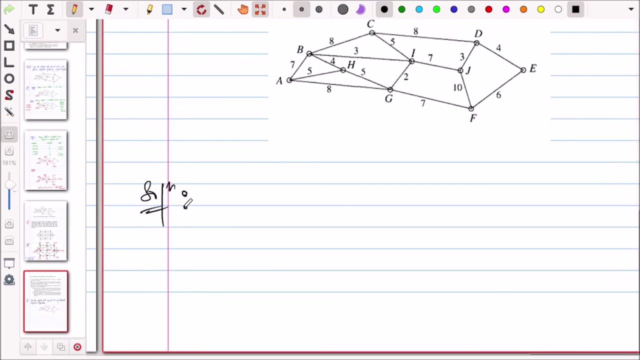 the same graph which we took earlier. so question: find the shortest path from a to e using improved extras you algorithm. so this is the graph. okay, so let us solve this. we label so at the start, a equal to V 1 is given permanently. we can use all the values to. 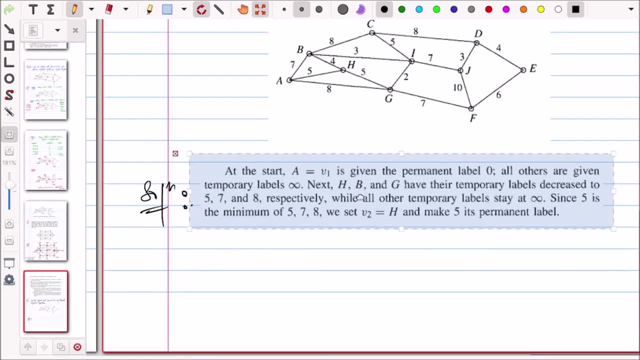 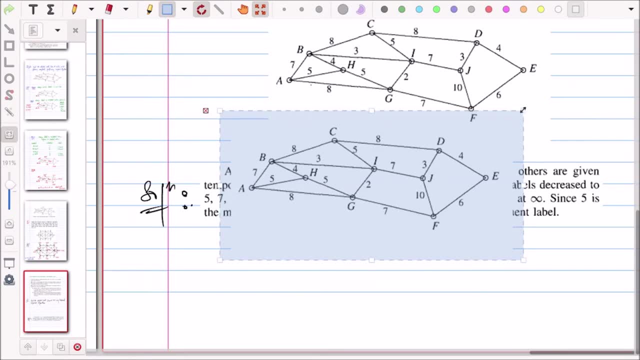 get the answer. so let us just go over this. we will take a sample starting. we will kind of write all these values right at the beginning. we will. V1 is given permanent label. this is the graph. so at the start A. so we will give permanent. 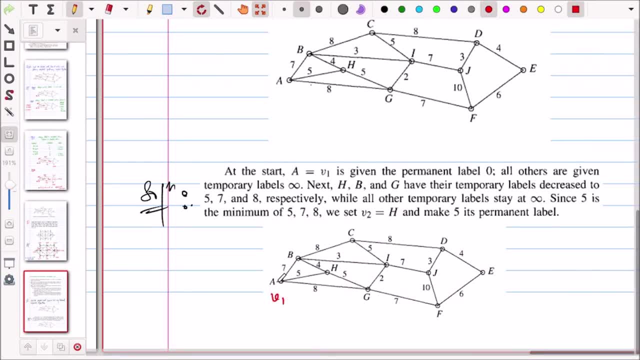 label to V1, V1 is given permanent label to V1 and this is given 0 label. this is called V1, this vertex is called V1 and we have given it a permanent label, 0.. Now next is: this is given in one step. rest of the temporary labels are infinite, so this: 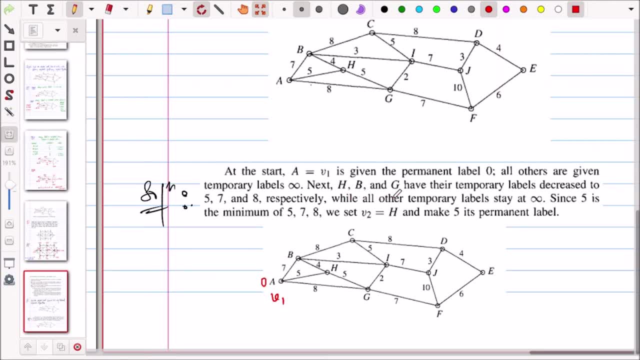 is permanently given 0.. Now what will happen is next: we will find all the vertices which are adjacent to A. so adjacent to A is VHG. so we have given it a temporary label 5, so we give it a temporary label 5.. 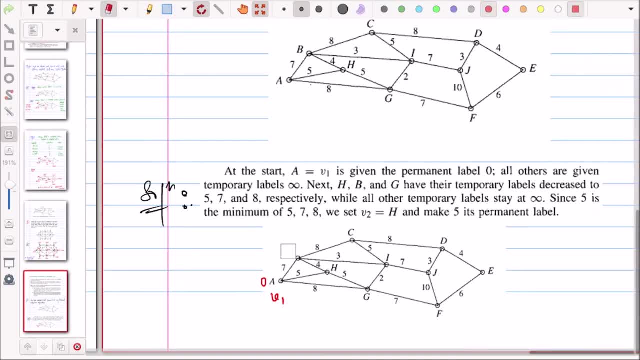 This is its temporary label, Sorry. its temporary label of B is 7, its temporary label of B is 7, its temporary label of H is 5 and its temporary label of G is 8, and rest of them are infinite Now, since 5 is the minimum now, which is the minimum of these three, 5.. 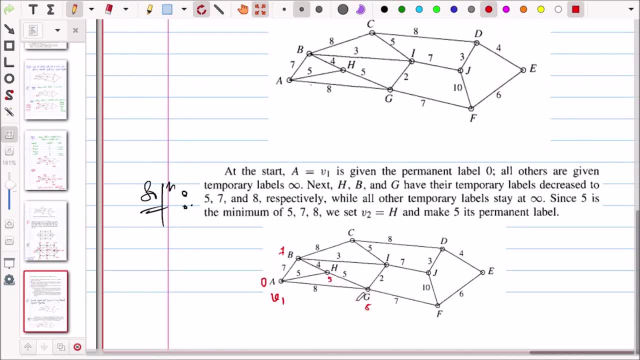 So we will just give the label to 5 and remove the rest of them. so this is its 5, so we have given V2 to this 5.. This is its permanent label. So we have given V2 to this 5, now we have called it V2 and made it its permanent label. 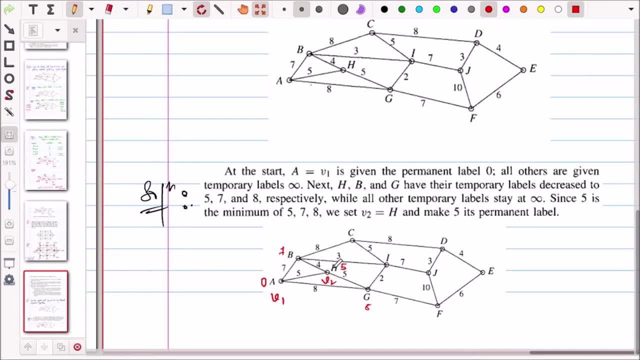 Its 5 is its permanent label. These are temporary. 7 and 8 are its temporary labels and its 5 is its permanent label. Okay, Is it clear? So now we are choosing the minimum one in every step. First we were labeling everyone at the same time. now we are not labeling everyone at. 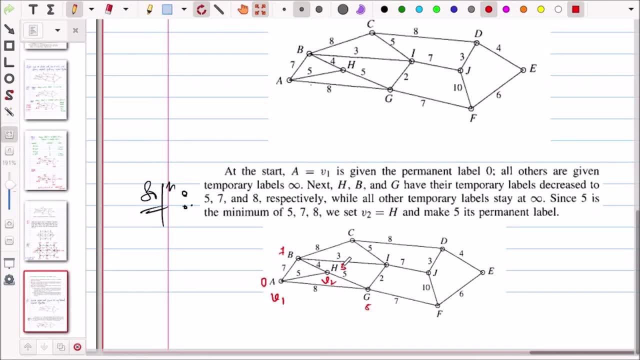 once. we are just labeling the minimum one. So this is its V1 and this is its V2.. Now, let us put the minimum one in each step. us go to the next step. okay, let us go to the next step. so now we will examine those vertices with: 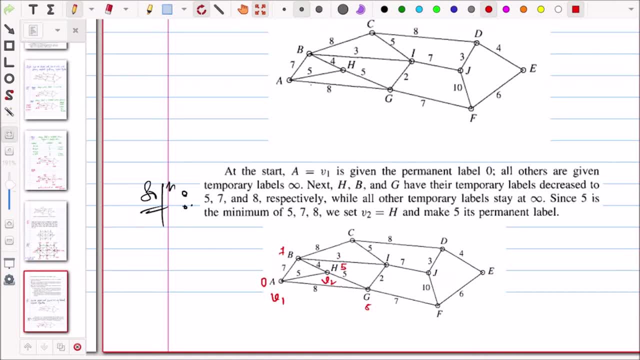 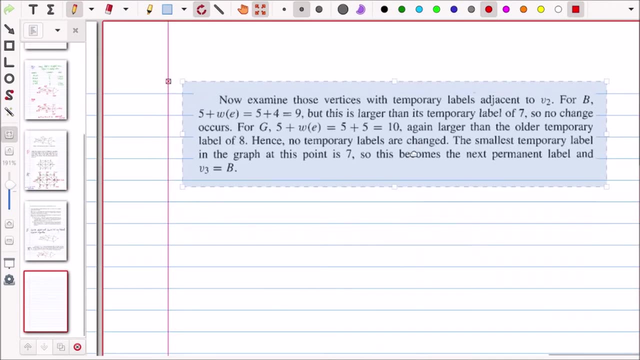 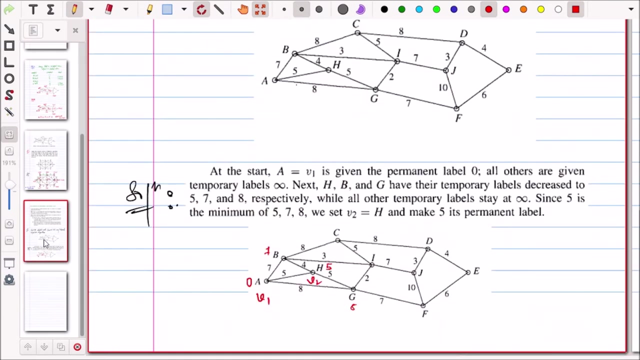 temporary level adjacent to vertices b. okay, so you will understand it. so this is seven is, its, eight is temporary. so seven, eight is temporary, v two and this is permanent. so even just go, we. i mean that is permanent and other labels are temporary, or back is up to infinity. 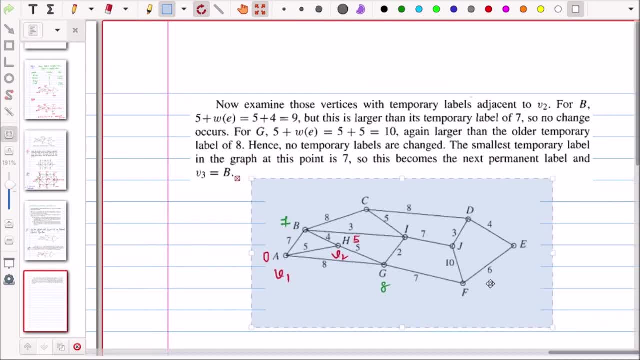 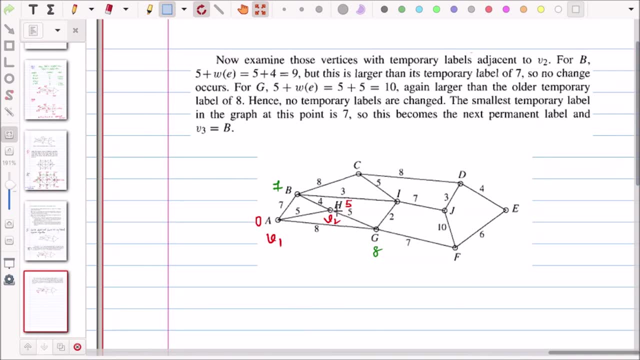 so now what will happen? yes, ah, um. yes, five plus four, so nine is greater than seven. okay, so this, which is larger than, because five plus four is nine, but this is larger than its temporary level of seven, so we will not change this temporary level. again, if you look at this, five plus five is ten, so it's the temporary level eight. 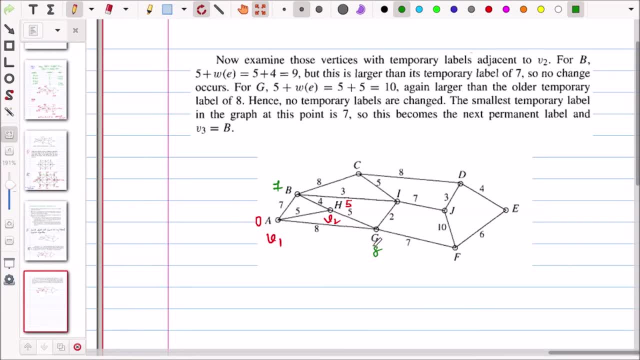 which is again greater than the older temporary level. so we will not change the temporary level, so it's seven. it is seven, so it's permanent. we will make this permanent permanent, so we will make it permanent. so we will call it v3, v3 and it's the permanent level seven. okay, is it fine? 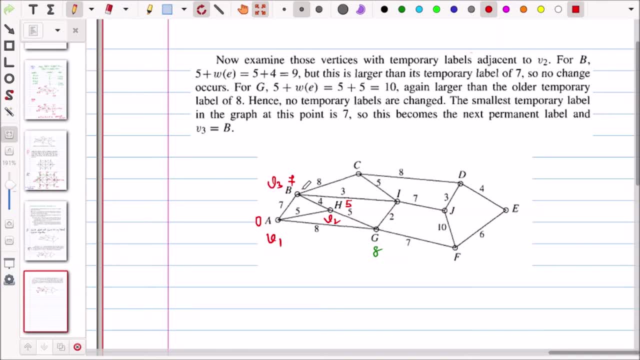 is it fine, okay, um, now. next we will come to this up because we will look at the neighbors of this. plus temporary label, right, oh, sorry, yes, i is also there, so c and i are the same i- these two vertices, will receive the temporary level in the next step. or message permanent. 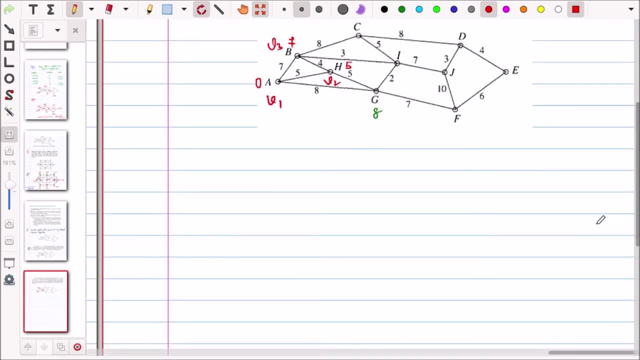 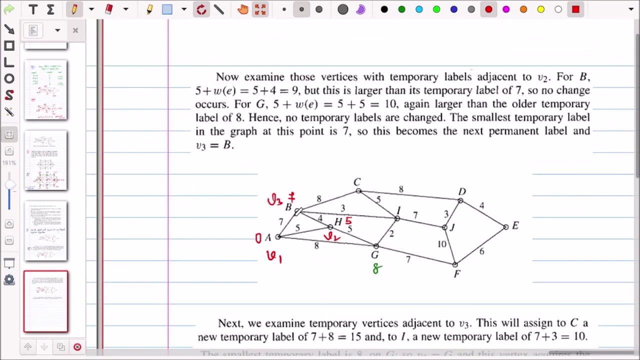 label. next we examine temporary vertices adjacent to v3, which is c and i. okay labels. check you can, because you don't have two different colors. so, like you have done in the book, you can circle it whatever is getting permanent. circle it, okay, circle that label whatever. 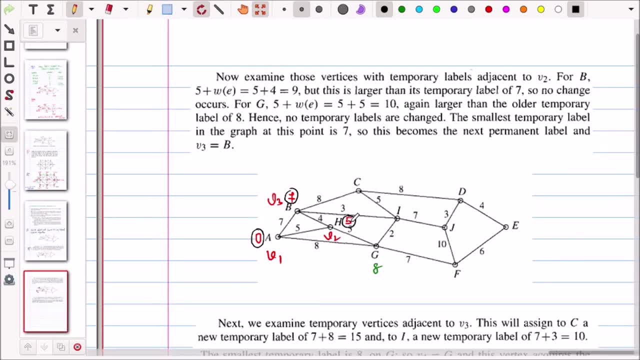 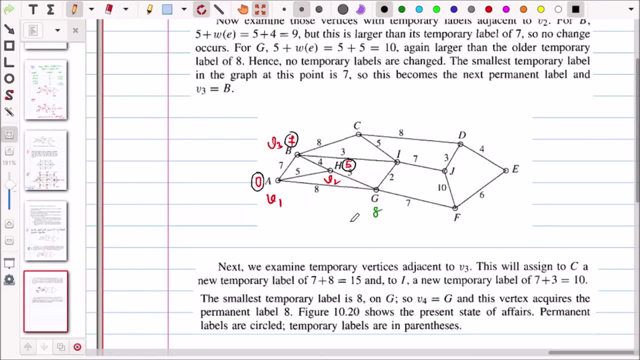 is getting permanent, circle it and those which are temporary, keep them like this, okay, because you don't have two different colors. you will not have two different colors. you will not have two different colors in the exam. so what you can do is you can give the circle. 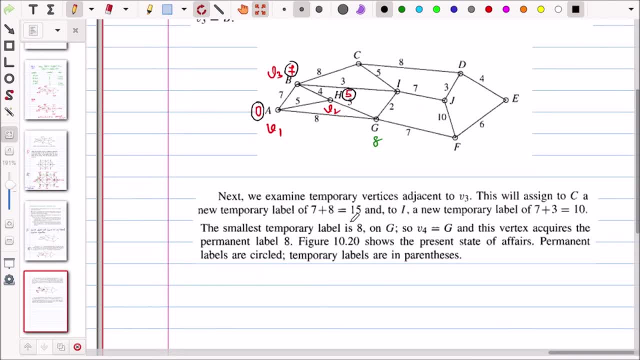 the labels with permanent color. oh, permanent label. okay, so c is seven plus eight, fifteen, okay, or it will come out to be seven plus three, ten, and which one is smaller? or a temporary level, okay, eight. so now we have three temporary labels. this is fifteen, this is ten, this is eight. 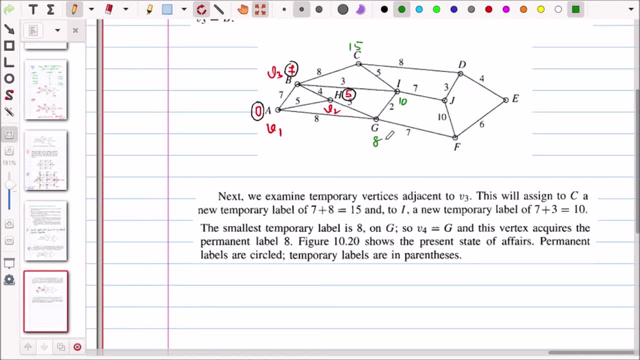 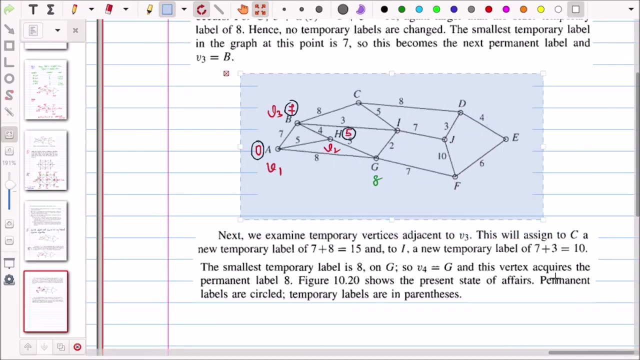 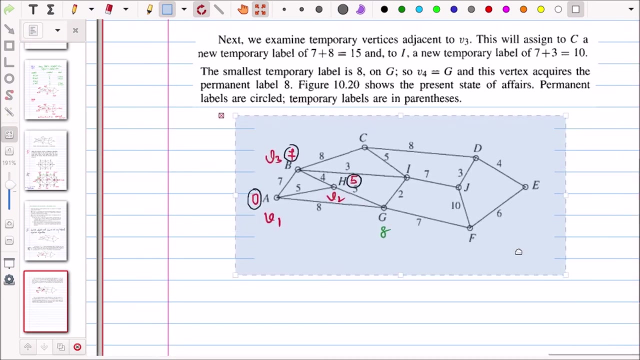 okay, so there are three temporary levels- fifteen, ten and eight- and which one is minimum? this is minimum, right, so this will be our v4, is it fine? okay? so, yeah, yeah, that will be good, this will be good. so this is 15, this is 7 plus 3, 10 and this is 8. so three different labels and because this is 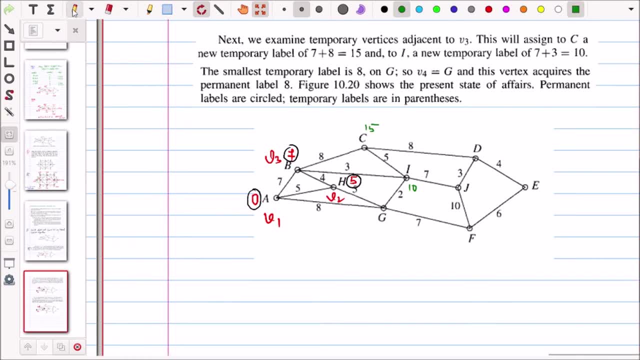 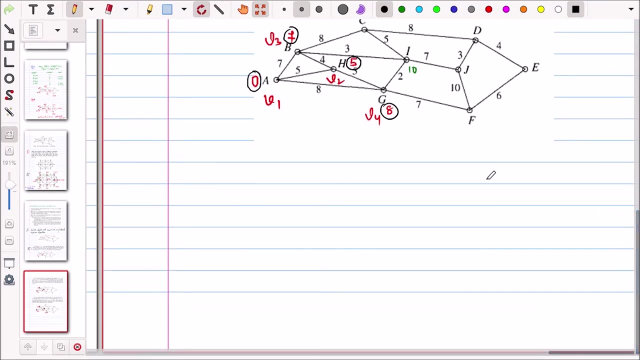 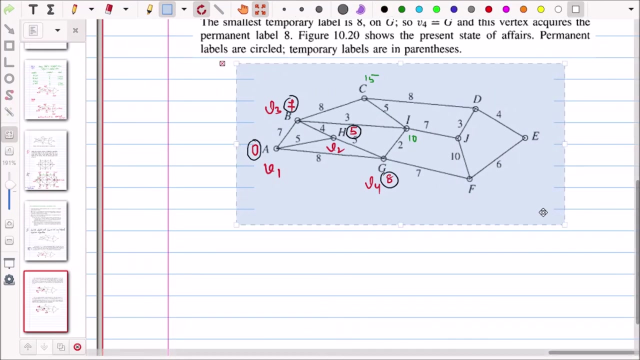 smallest. so this will become permanent label. so we will make it a permanent label. so this is our b4 and this is our 8. which is already there, and 8 plus 7, 15, right? so next label, which is 10. now we have two choices. 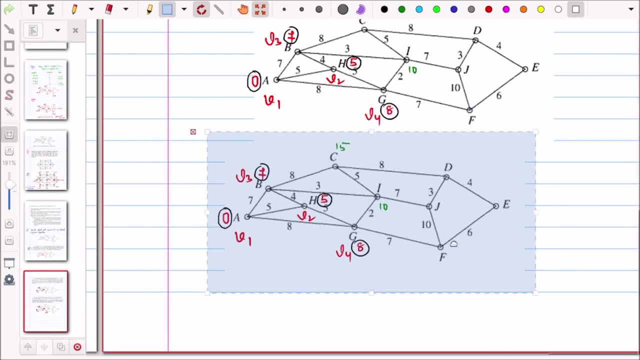 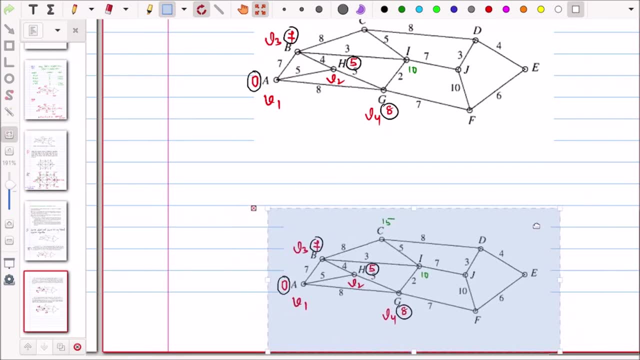 here is only one choice, so so i will make it permanent. this will become v5, v5, and its permanent label will be 10 and its temporary label is 15. this is also 15 and this is also 15. okay, is it fine? yes, sir. 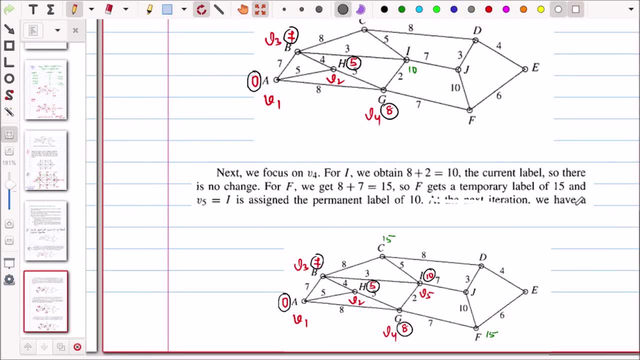 this is your, okay, so you can see. next we focus on v4, v4 then. then for i it was 8 plus 2, 10 and for f it was 8 plus 7, 15 and c was already 15. so again, minimum is: 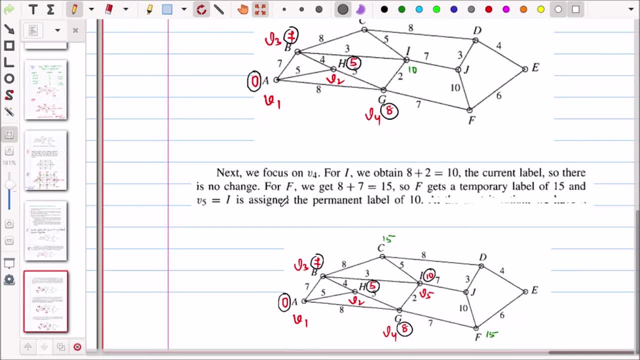 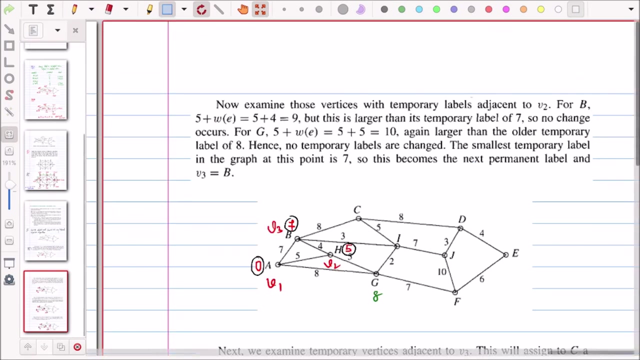 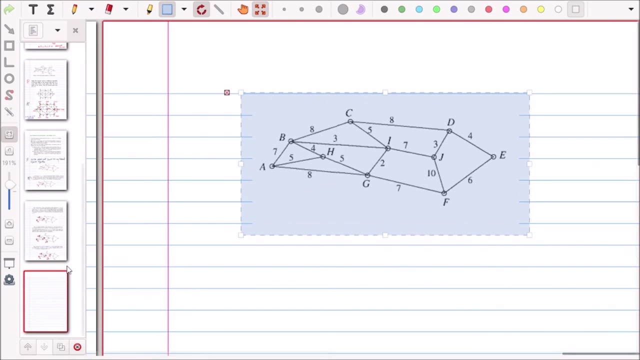 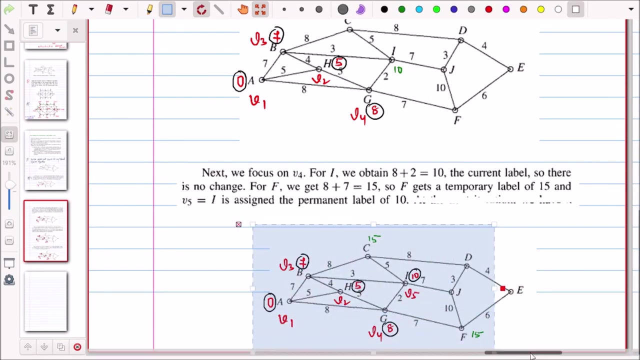 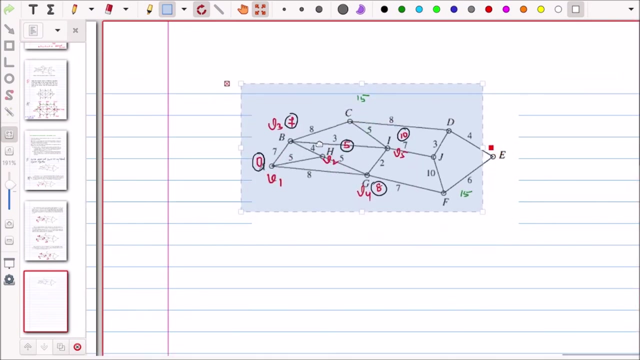 this 10, so i receives that permanent label v5 with the label 10 right up. next step is: so what? what are the the those 10 plus 7, 17 or c 15? yes, you, you, you okay, yes, because this is receiving the temporary label. 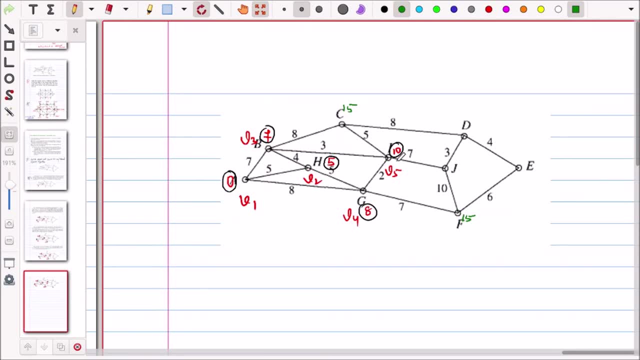 now j is receiving the temporary label 10 plus 17, 10 plus 5, 15, which is same, and any other vertex, no. so now these two: minimum concept, now 15. so this will be our v6, right v6. and what is the label? 10 plus 5, 15. okay, up next quickly recently, label attain correct. so we will. 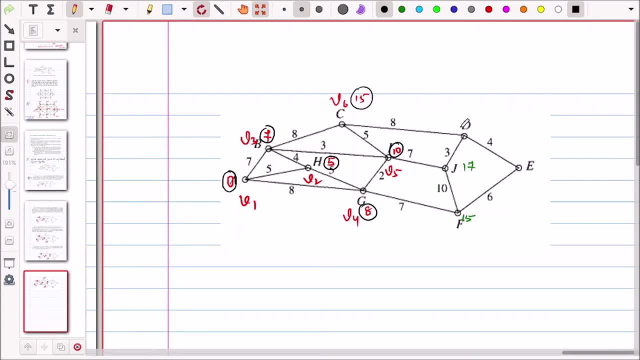 see, what is this adjacent to this, which is 15 plus 8, 23? okay, so this will receive 23 label. this is 17, this is 15. so which one is minimum? 15, 15. so we could have gone for f or we could have gone for. 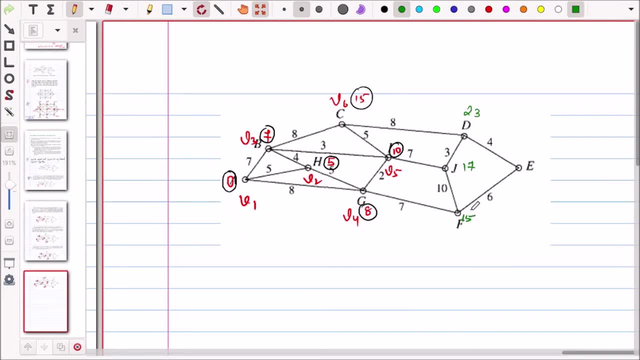 uh, c, so c step, which is the minimum f, right? so yeah, this will be v7 and this will become permanent. okay, he 17, then he 17. so No, it's easy. yes, he should. even. yes, okay, fine, sure, next. so first matrix. so, if you can stand in the circle, 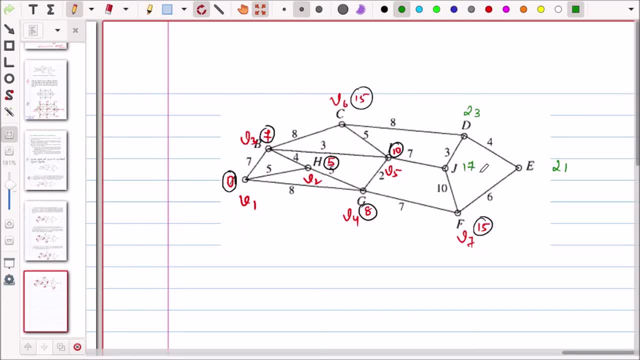 so this time, even in every twenty places, две is the main, second, technically same这个 property, the change over right. yes, is it right? so so this will become v8 and it will become 17, so now vertex, which is unlabeled, and distance. so yeah, yeah, my pass, or it's got 17 plus 3. 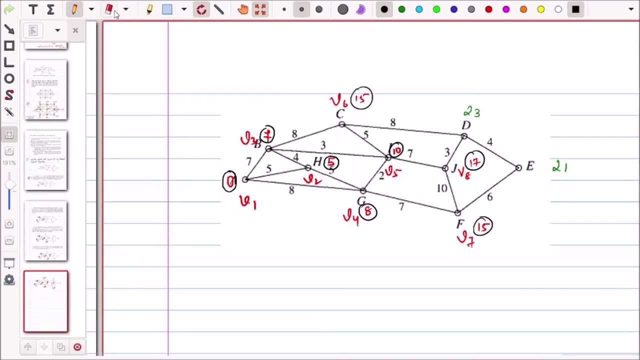 20. so yeah, they will change. this level will change. it will become 20. okay, this will become 20 and okay. so yeah, this will be v9 and this will be 20, okay, so, and this is your 21 ticket, Is it fine? 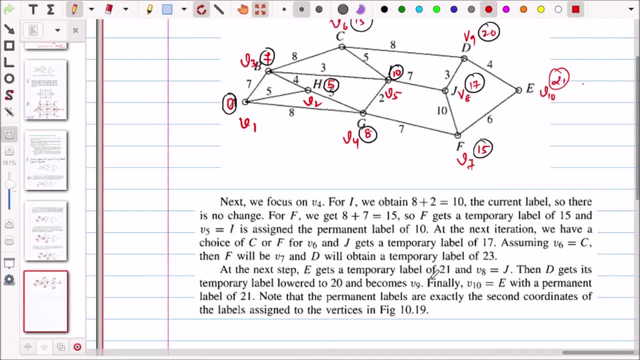 So this is all there. So you already take here. So he gets a temporary level 21, V8 is our, this J, and then D gets a temporary level lower to 20. So it becomes V9. And then we finally V10, with a permanent level of 21.. 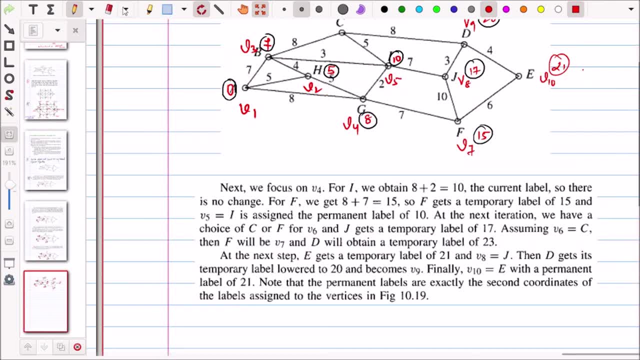 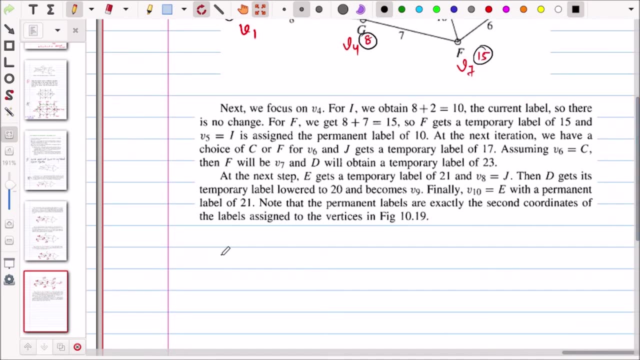 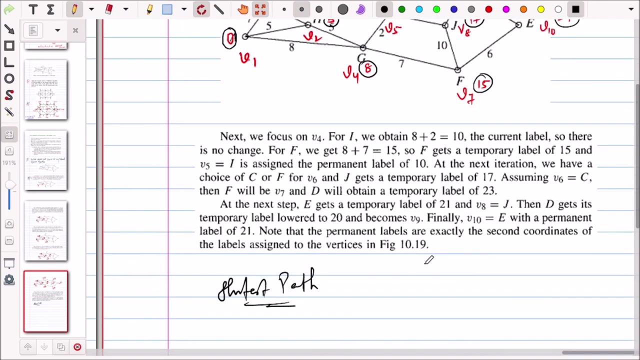 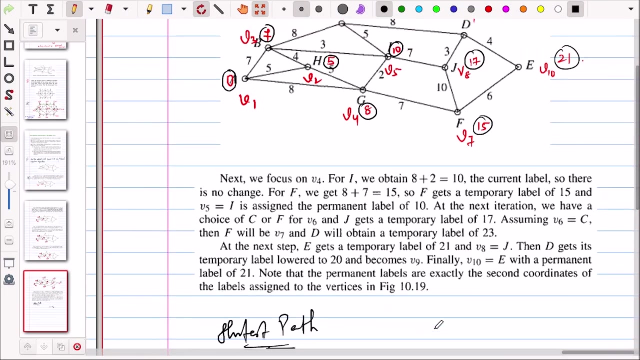 After this, can I walk this so classical, the path trace. So how about a short spot, Shortest path? Yes, if you look at this. So we can, We can- I'm constantly thinking We can from V7, right. 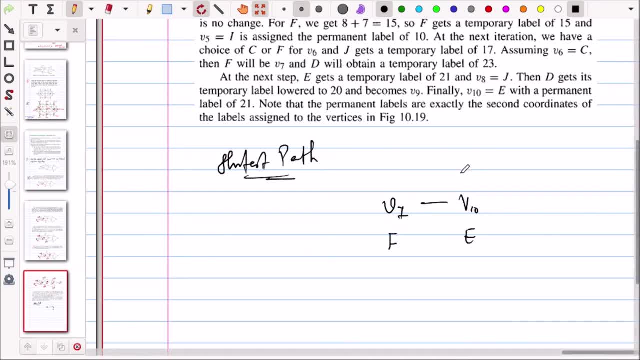 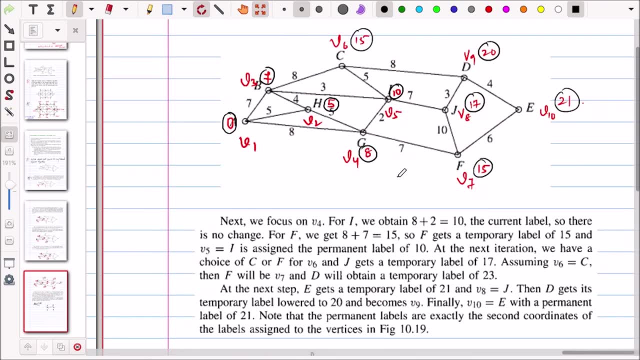 V7. so this is E, This is your F 21. 15. OK, now what next? I'll give 15 cancer, either 8 plus 715, right 8 plus 715. so, Joe, distance one right previous level car. why you see us pay down about this? 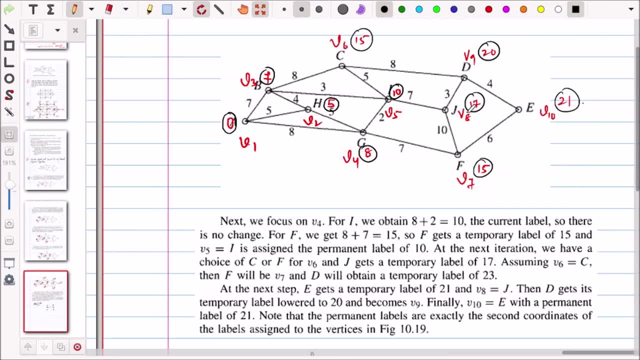 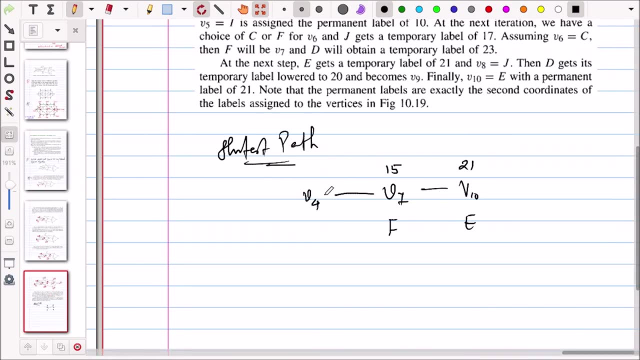 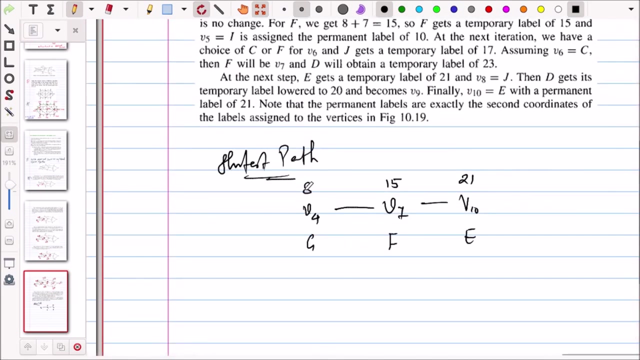 We will come out to be V4. so we'll come to V4.. Take it Before, so give me up a 6. so this is V4, which is your G Orosco level 8, the up 8 kiss era. if you look at this,